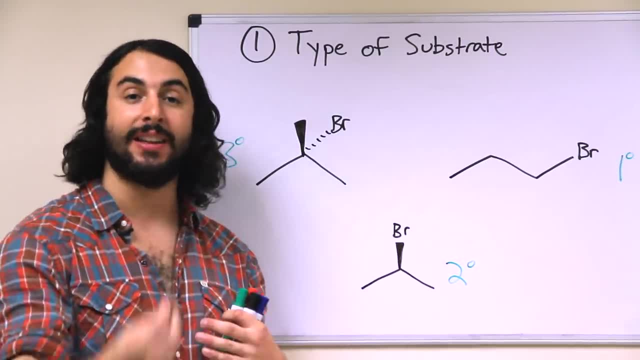 that's a lot of electron density that is going to repel any incoming nucleophile that is negatively charged. So with a tertiary halo alkane there's a lot of alkyl groups. that's a lot of electron density that is going to repel any incoming nucleophile that is negatively charged. So 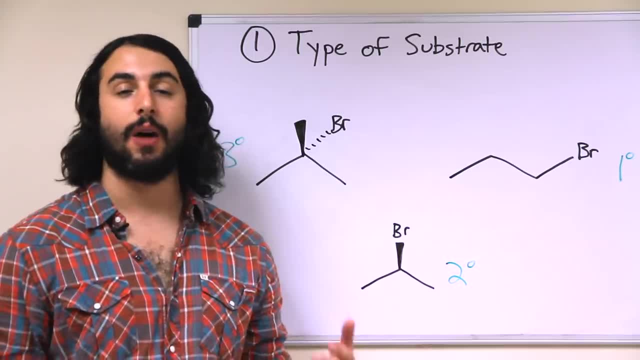 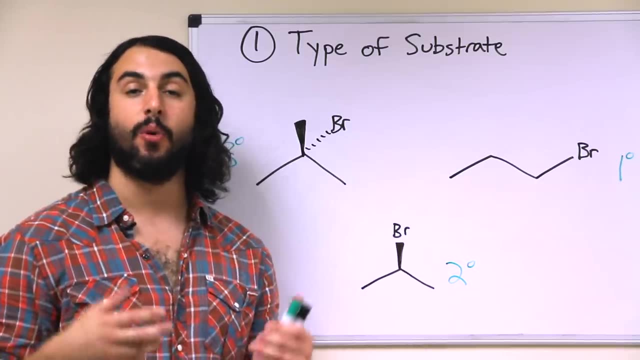 if we look at this tertiary halo alkane, we can rule out SN2, that's not going to occur. However, SN1 is a very good candidate because we know that the more substituted that a carbocation is, the more stable it is due to the hyperconjugation from the neighboring alkyl groups. 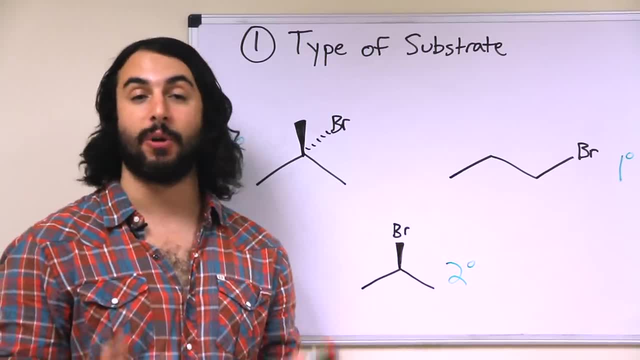 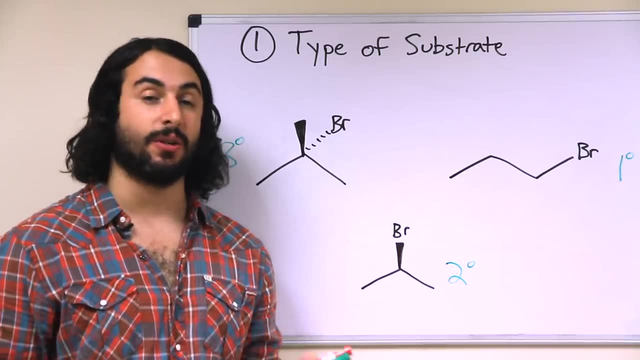 So if this bromine were to leave, it would leave a tertiary carbocation which is stable. so SN1 is a very good candidate. Therefore, E1 is also a good candidate and E2 is also possible. So basically, with tertiary, we know no SN2.. 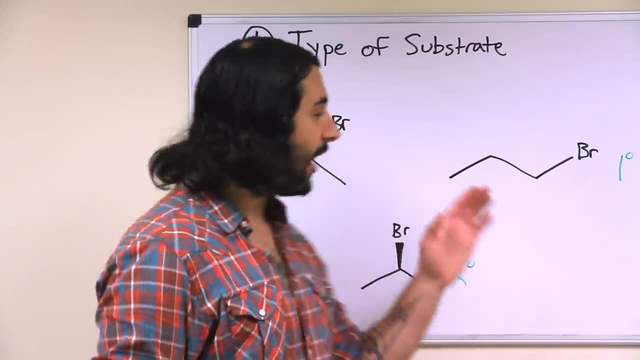 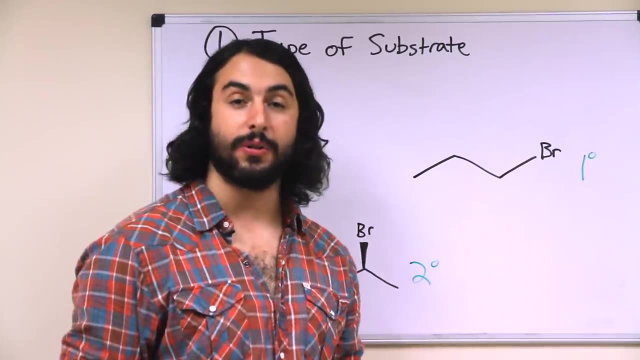 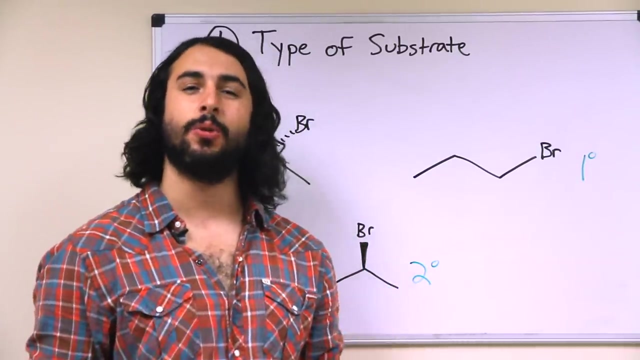 With a primary halo alkane. SN2 now is very possible. there's not very much steric hindrance. it's going to be very possible for a nucleophile to approach this carbon in this direction, And so SN2 is going to be possible. E2 is also possible. However, SN1 and E1 are very unlikely. 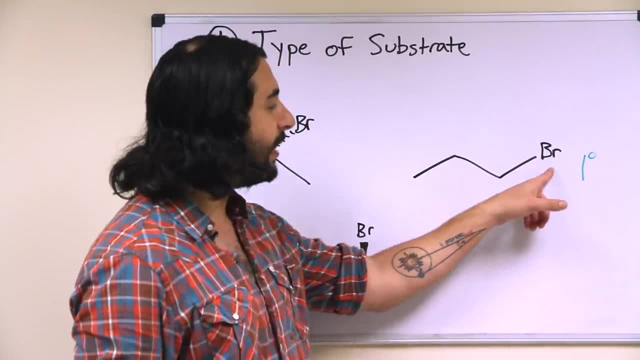 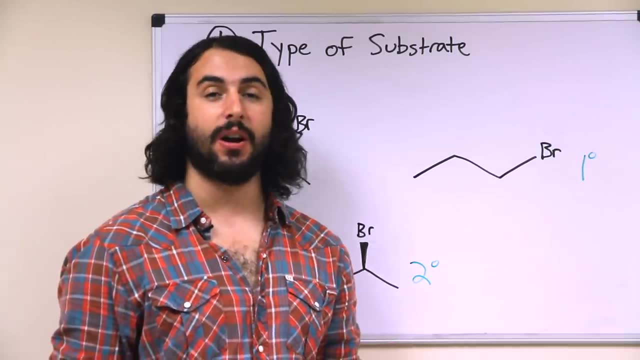 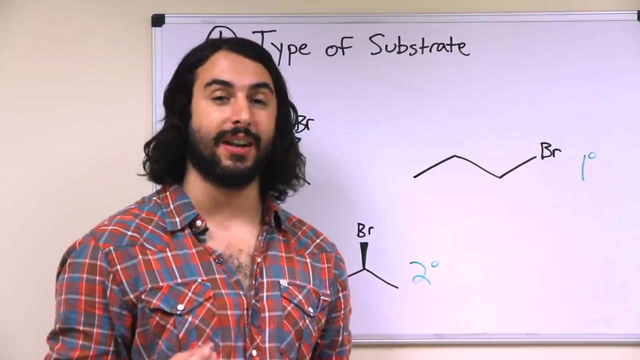 to happen because if this bromine is to leave, that would leave a primary carbocation. A primary carbocation is very unstable because it does not get to enjoy very much hyperconjugation from neighboring alkyl groups. So because a primary carbocation is very unlikely to form, we can. 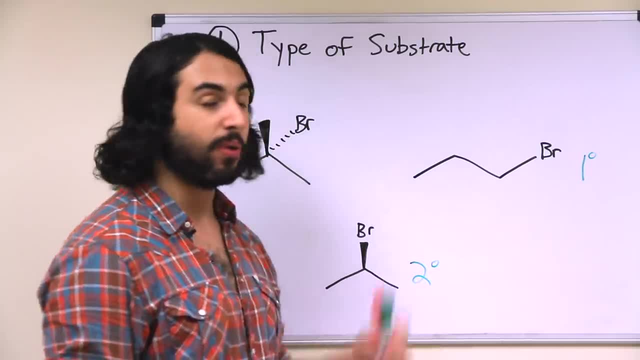 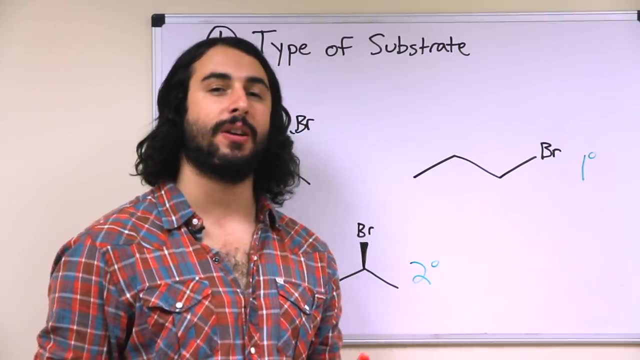 more or less rule out E1 and SN1 for a primary halo alkene. There are some exceptions, like an allylic system, but at this stage we can pretty much just take it for granted that a primary carbocation is very unlikely to form With a secondary halo alkene. there's not that much. 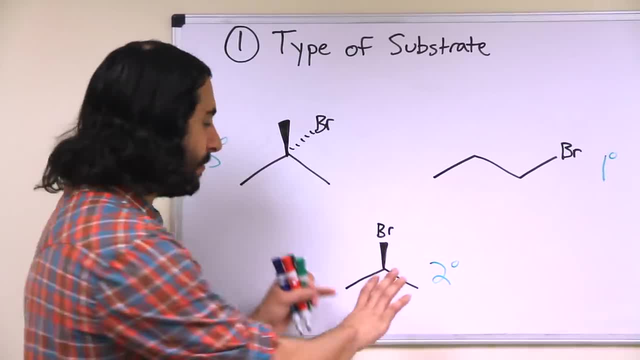 information that we can get. If there's a lot of beta bromine, there's not a lot of beta bromine, there's not a lot of beta branching or some steric hindrance, more towards the sides, that might be a factor in repelling a nucleophile that's going to do SN2.. 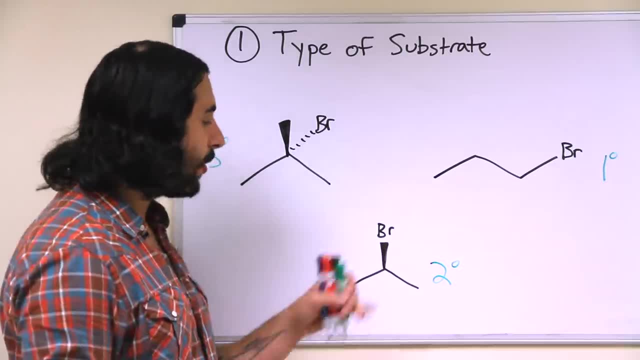 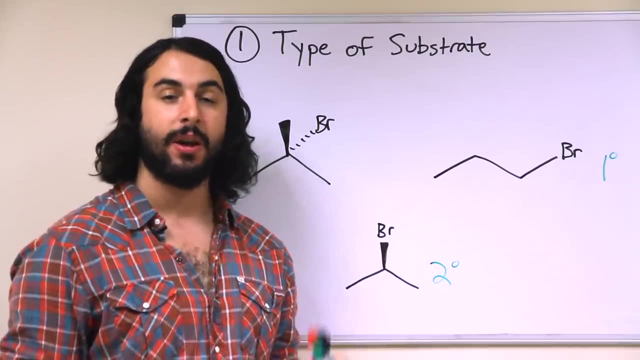 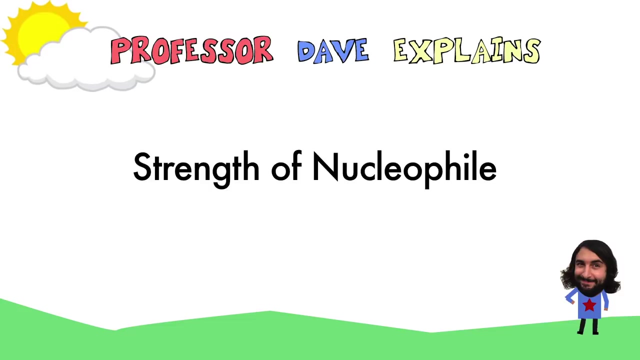 But basically with a secondary halo alkene we can't really gather that much information about what mechanism is going to occur just by looking at the substrate. But for tertiary and primary we are able to rule out some possibilities. The next thing we want to look at is the strength of the nucleophile and leaving group. So the first 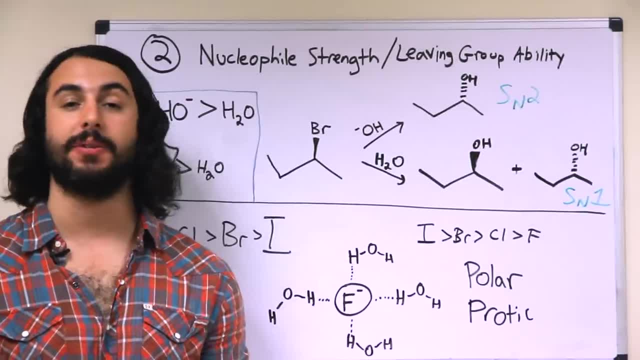 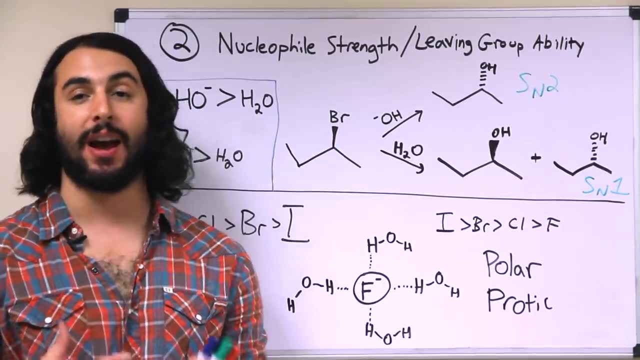 thing we want to look at is the strength of the nucleophile and leaving group. So the first thing we want to understand is that nucleophilicity parallels basicity. This means that there's a correlation between how much a group is able to coordinate to a proton and how well a group is. 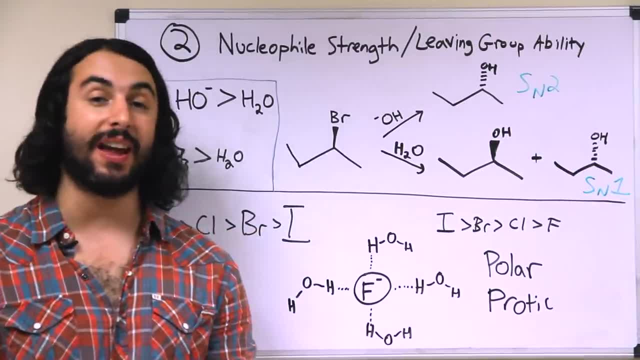 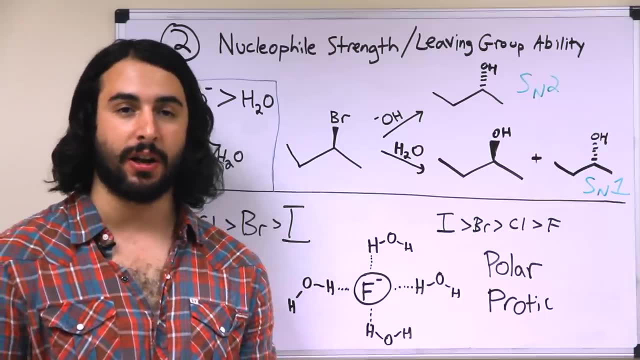 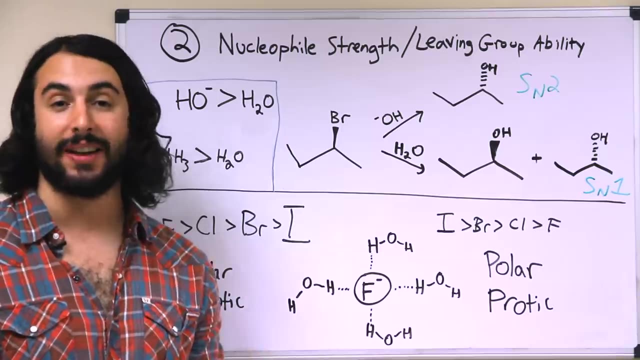 able to coordinate to a molecule. So something that's a very strong base seeks to form a bond to a proton, but it could just as well act as a nucleophile and coordinate to a molecule. So, for example, hydroxide is a much stronger base than water. It has a 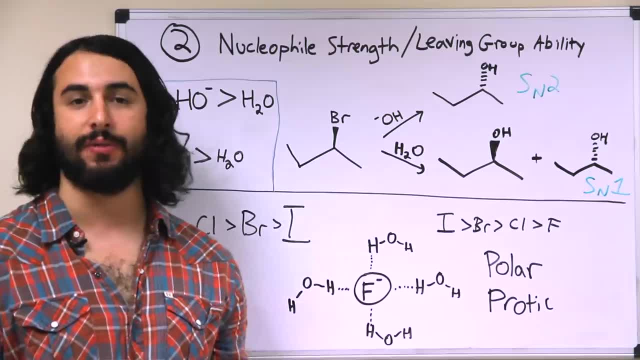 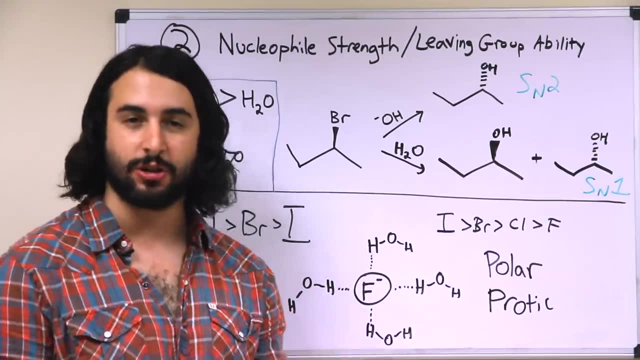 formal negative charge. It's a strong base. A water molecule is not very basic. In fact it's neutral. So that means that if let's say, we keep it real simple and we're just trying to decide between SN1 and SN2, we'll take a look at the eliminations later. If we look at this, 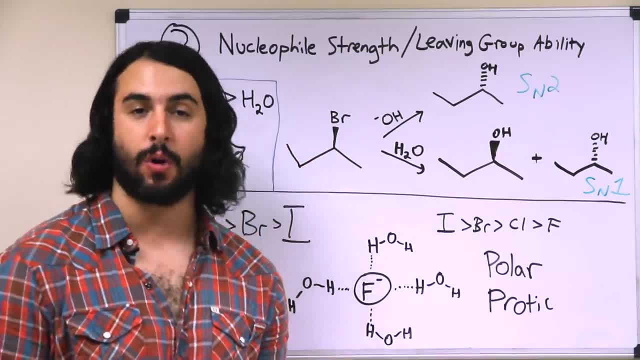 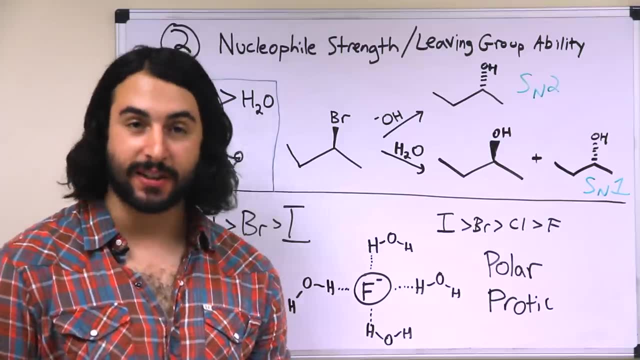 substrate and we look at what would happen whether hydroxide or water were to attack. now the hydroxide is a very strong base, So it's a very strong nucleophile, So it is capable of an SN2 reaction. So there's the SN2 product. However, a water molecule is not strong enough to do SN2. 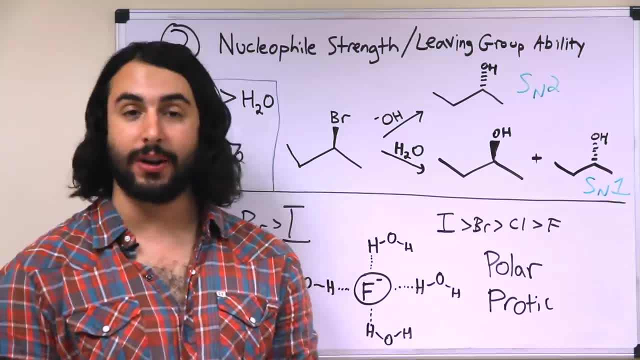 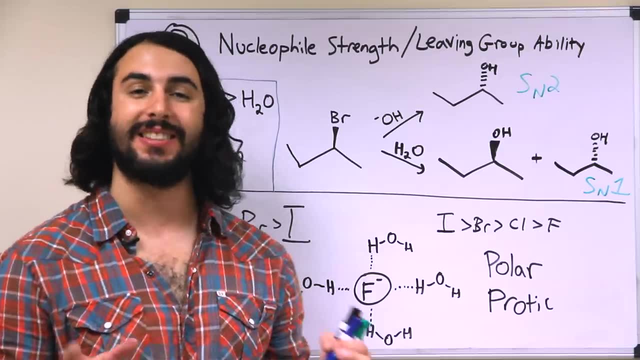 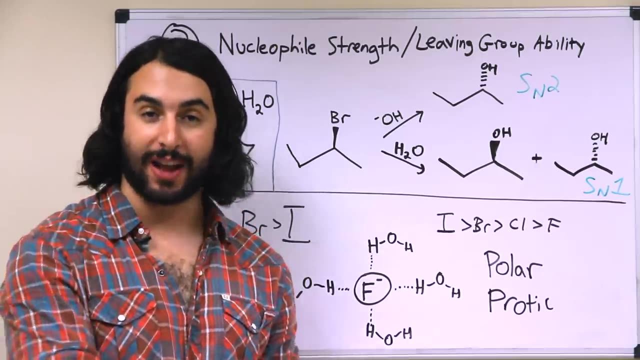 It's not a strong nucleophile, So but what could happen is that if the bromine leaves, leaving a carbocation intermediate, that is a very unstable situation. So a water molecule would be a strong enough nucleophile to coordinate to a carbocation and then deprotonate. So 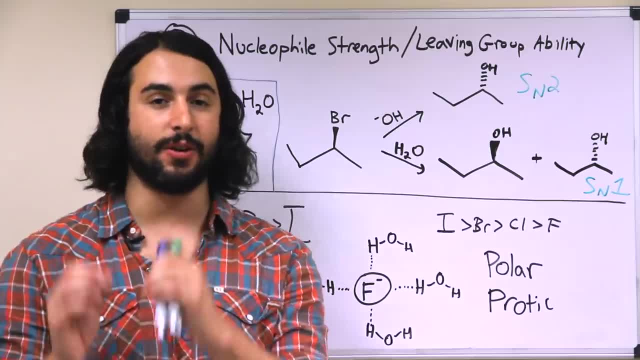 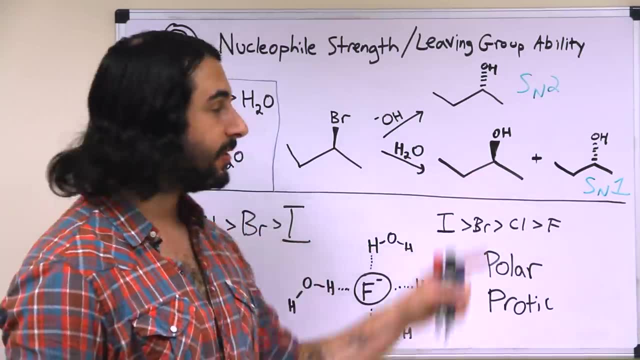 basically, a water molecule is capable of behaving as a nucleophile in an SN1 reaction. Recall that if we do an SN1, we're going to get a racemic mixture. So there's the two enantiomers. So that's the main takeaway We want to understand. 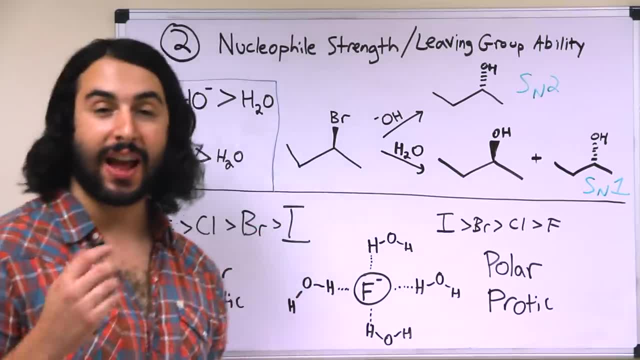 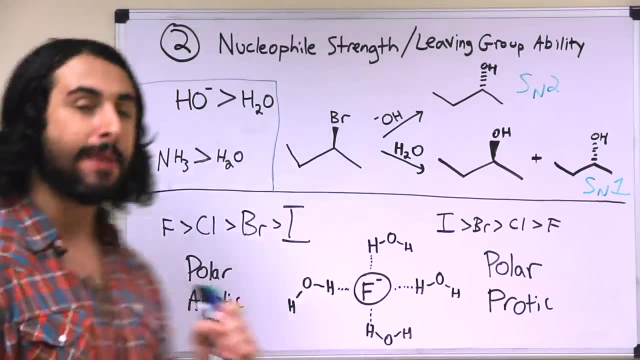 that nucleophilicity parallels basicity. Now the halides are going to be very common nucleophiles as well as leaving groups, So we want to understand how those behave. So in a polar aprotic solvent- meaning the solvent does not have any protons that are available for- 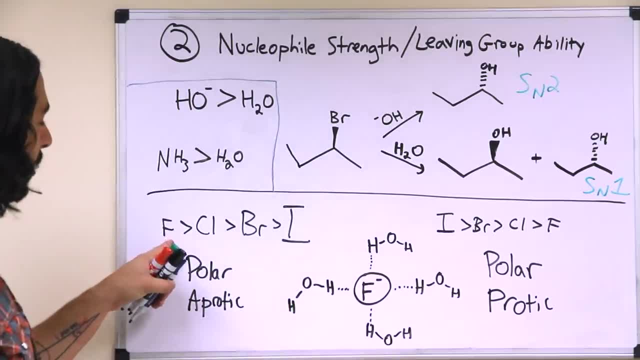 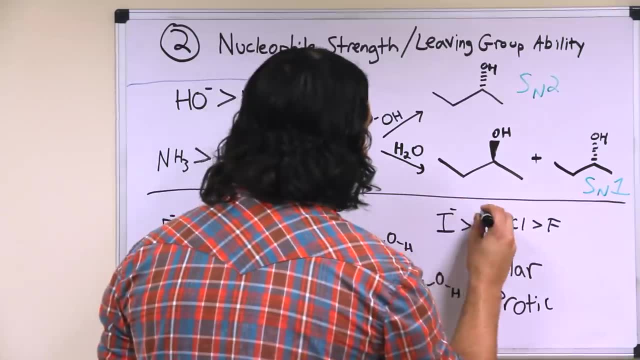 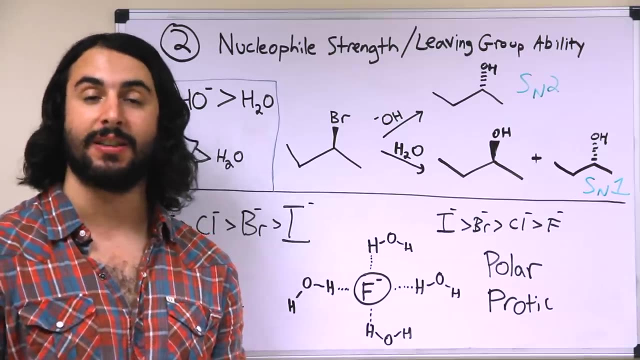 dipole-dipole interactions. it is going to be the case that fluorine- or I should say fluoride- let's make these all the anions- the fluoride is going to be the strongest nucleophile because it is the strongest base of the halide ions. So the reason for that is that as you go down the 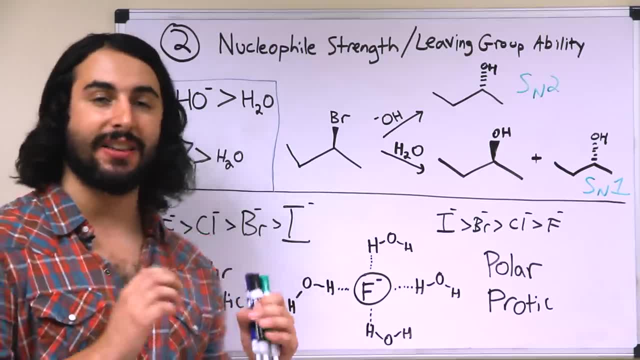 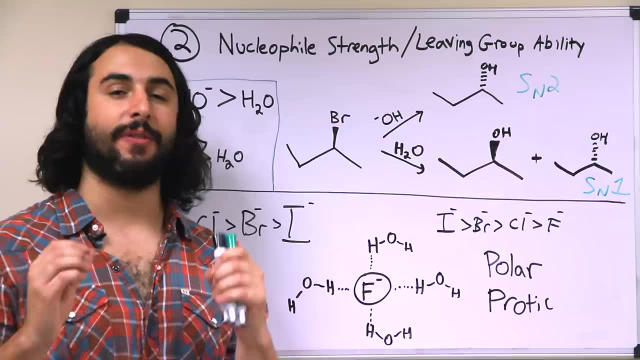 periodic tables. you go down the halogens, the ionic radius is getting larger as we go, and if we have a larger ion then that becomes more polarizable. So what that means is that it's a larger volume reaction in cause, that it is stronger, So we're keeping the climate going. 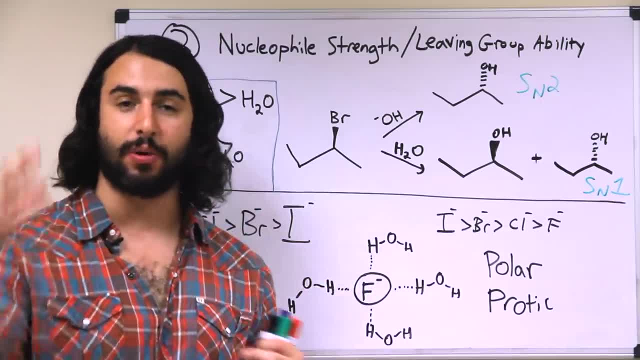 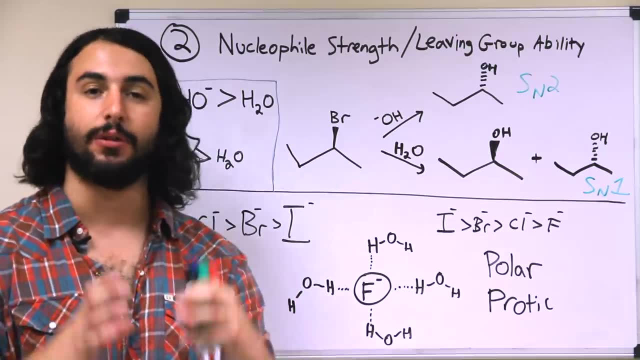 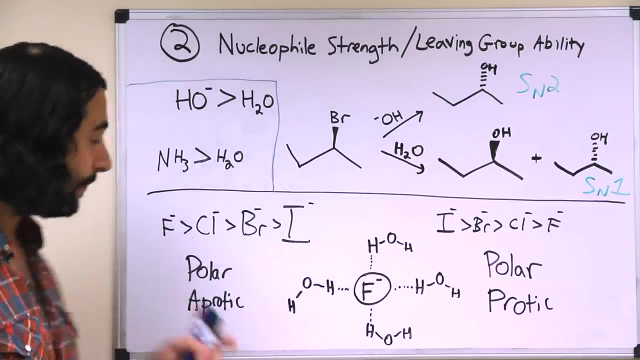 okay, with which that ion can diffuse and spread out its negative charge. so because the negative charge on the fluoride is highly localized on a very small ion, that makes it a very strong nucleophile. now all the halide ions are good nucleophiles, but in a polar aprotic solvent it's going to be fluoride. 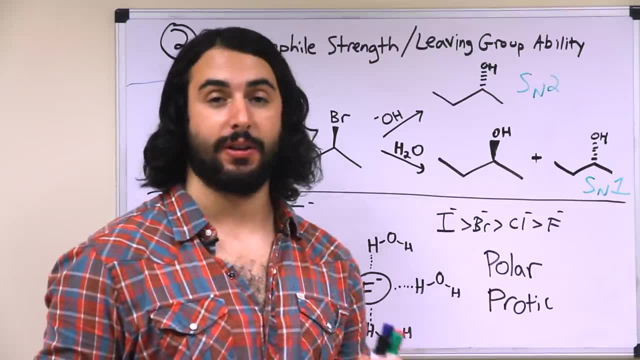 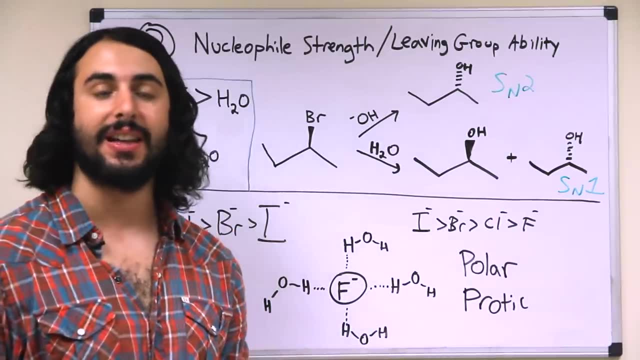 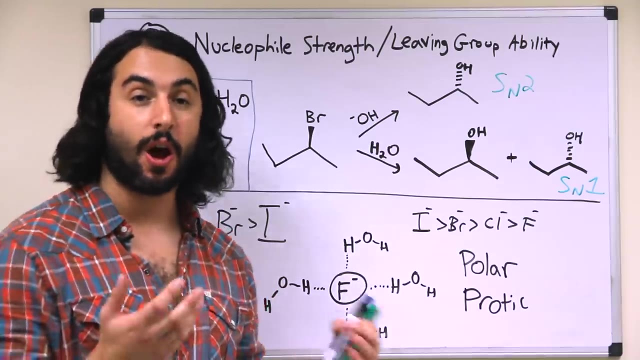 that's the best. now, if you're looking at a polar protic solvent, this trend is going to reverse because, by the same token, if the fluoride is much more basic, that means that it's going to spend the most time in solvent interacting with any available protons, let's say the protons on a water molecule. so we can. 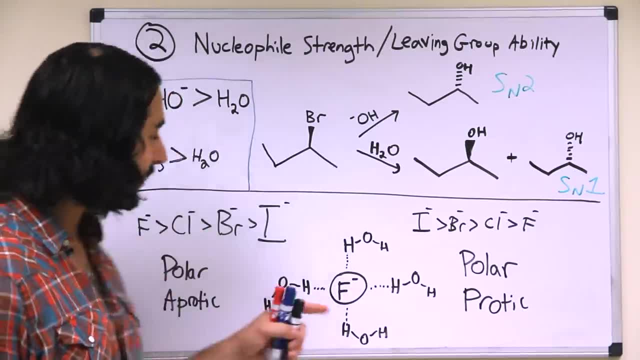 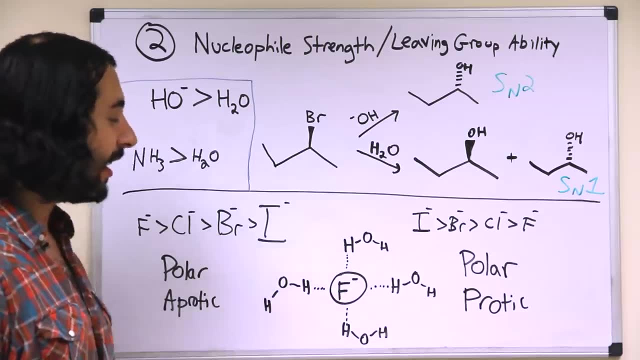 see here. so water is a polar protic solvent, right, because these protons are available for ion-dipole interaction. so this is an ion-dipole interaction and there are several that the fluoride ion is able to participate in because it has a very localized charge. 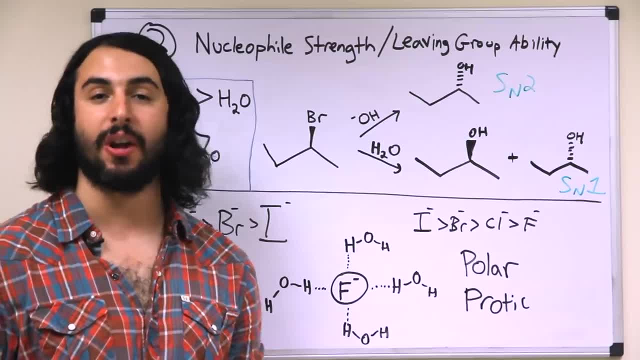 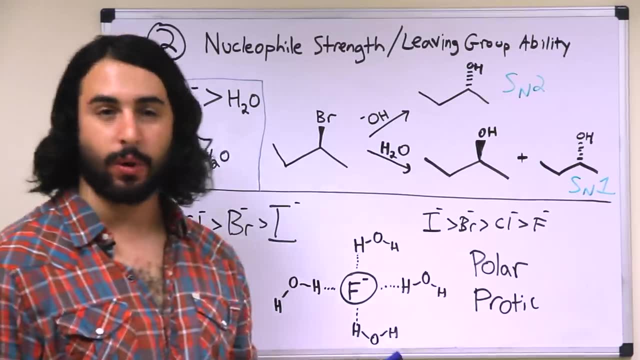 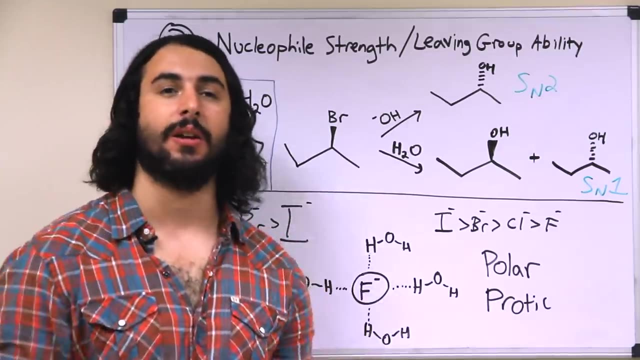 so because the fluoride ion is spending much more time interacting with molecules of solvent. that is going to hinder its ability to act as a nucleophile, whereas it still will be able to. but in this case the iodide is going to be the best because its charge is more spread out. it's more 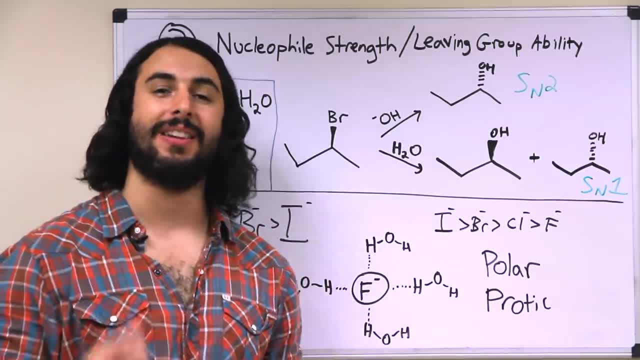 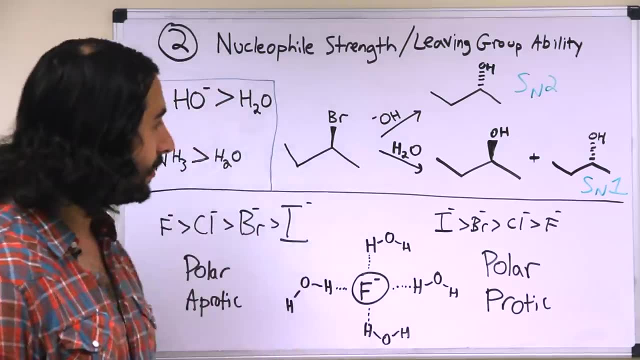 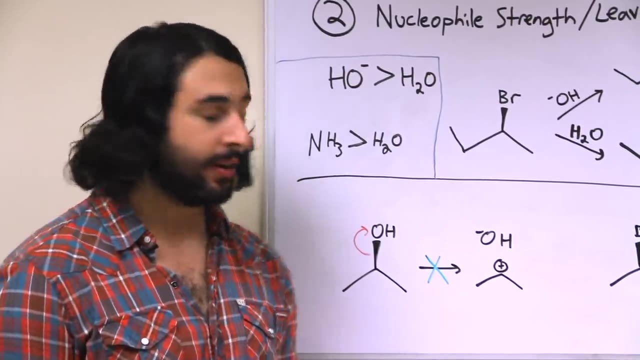 diffuse. it's more polarizable, so it is going to be spending less time participating in interactions with molecules of solvent, which will make it the best nucleophile of those. so leaving group ability is basically the opposite side of the coin. so it's precisely for the same reason that hydroxide is a very, very strong. 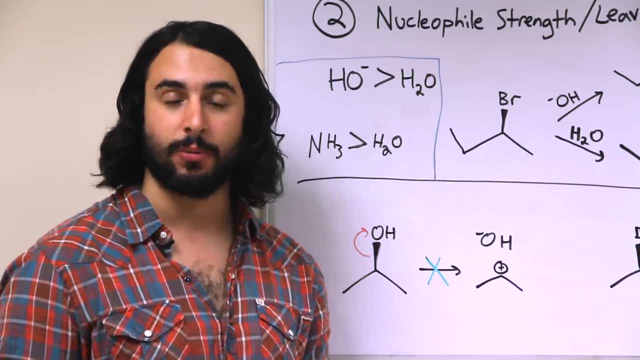 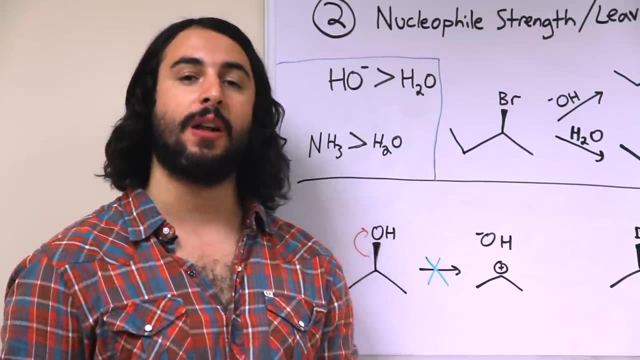 nucleophile. that's the same reason why it's a terrible leaving group. so hydroxide is very basic. it's unstable. it seeks to coordinate to something, so it should follow that if it's such a good nucleophile then it's not really going to. 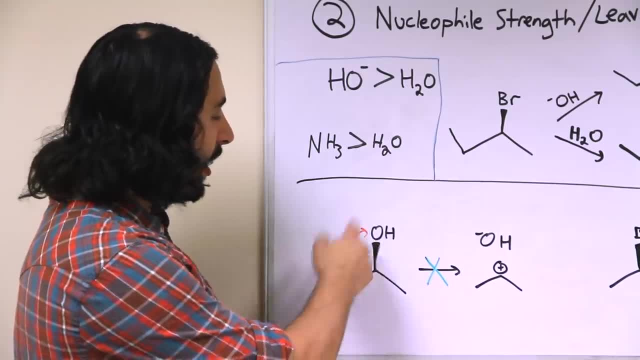 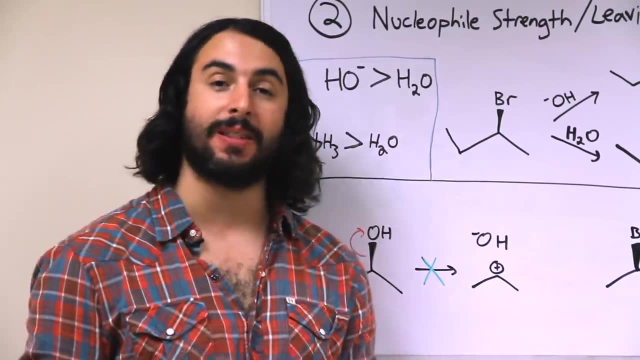 be in a rush to leave. so that's why a hydroxyl group is a good nucleophile is going to be a bad leaving group because it's so basic. now, however, if we tack on another proton to make that a water molecule, water is a very 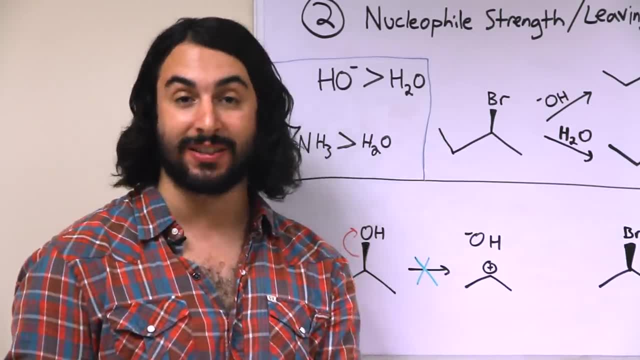 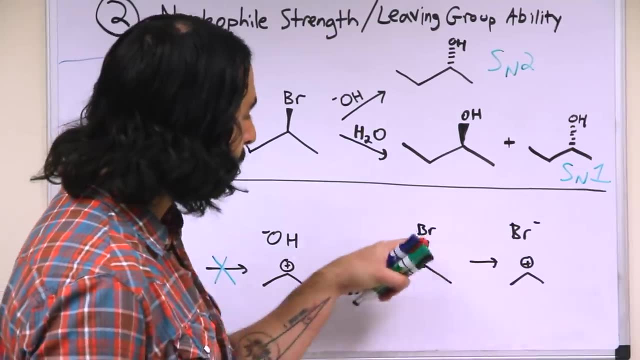 good leaving group because a water molecule will be very stable once it has left. so that's why the halides as well are very good leaving groups, because bromide is perfectly happy on its own. it's got a full octet, so that's not. 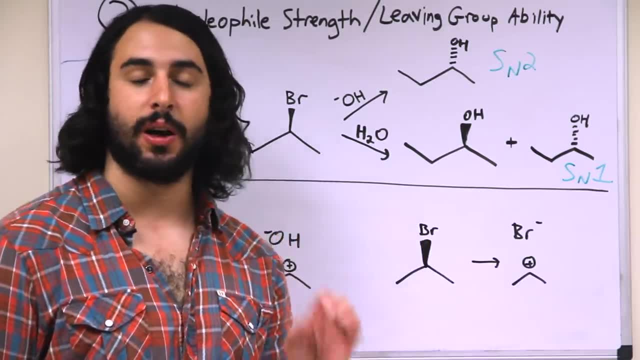 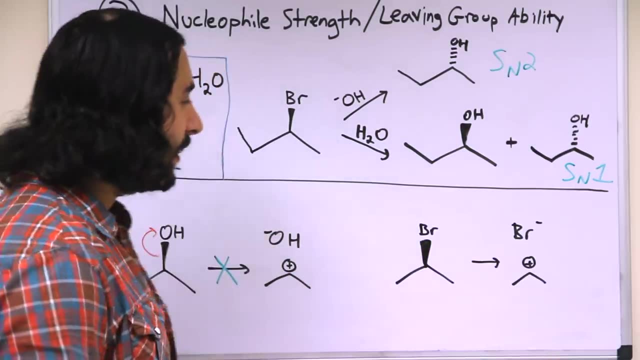 going to be a problem and we can look at the same rules with which we examined the nucleophilicity of the halides to examine which ones are going to be the best, leaving groups, because we can see, depending on whether it's a polar protic. 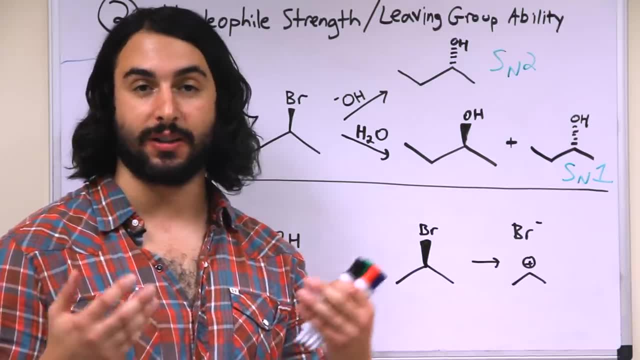 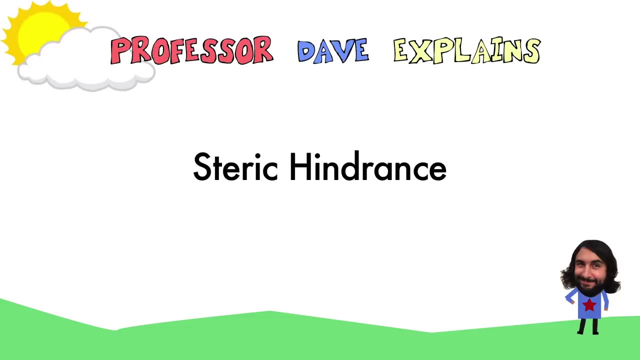 or a protic solvent. we'll know how well it is going to interact with the protons and solvent so, but those are all going to be pretty good leaving groups. a third thing that we want to look at is the steric hindrance associated with the. 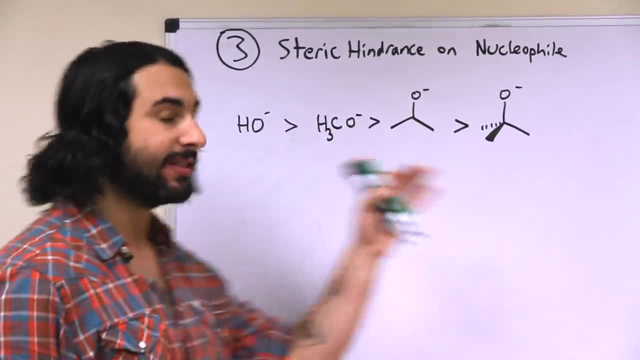 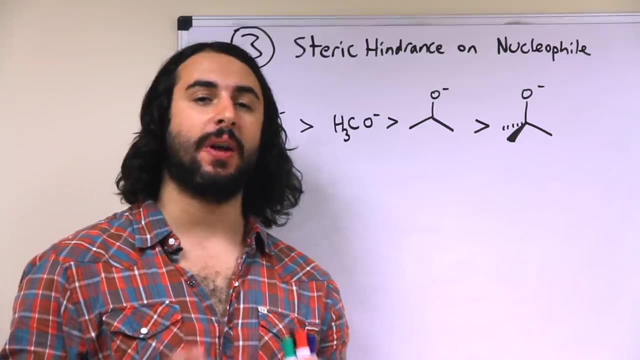 nucleophile. so let's take a look at these: the hydroxide and some alkoxides, so these all have a lot to do with the nucleophilicity of the nucleophiles. so we all have O minus as trying to behave as a nucleophile. so we have roughly the. 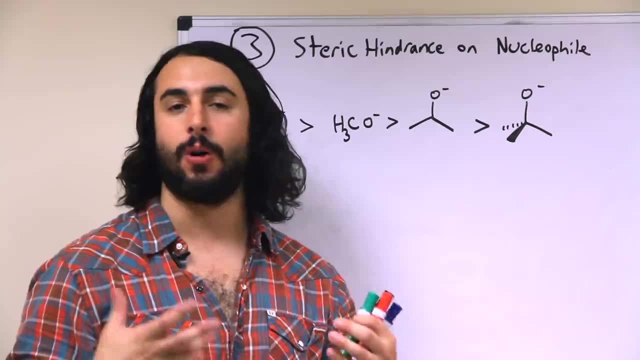 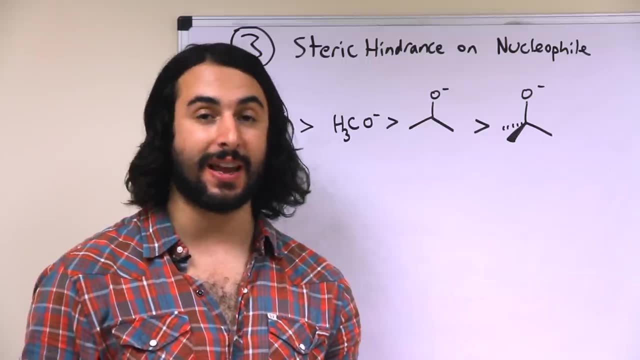 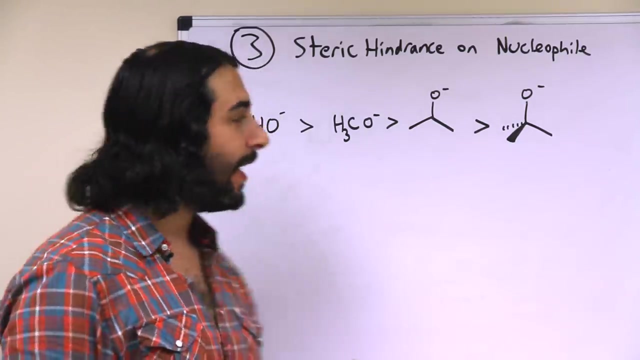 same basicity there's. there's a small variation, but it's all O minus, so there's not much difference in the basicity here. so technically, the nucleophilic strength is roughly the same. however, look at what's happening: as we are adding more and more carbons, branching. this is increasing the 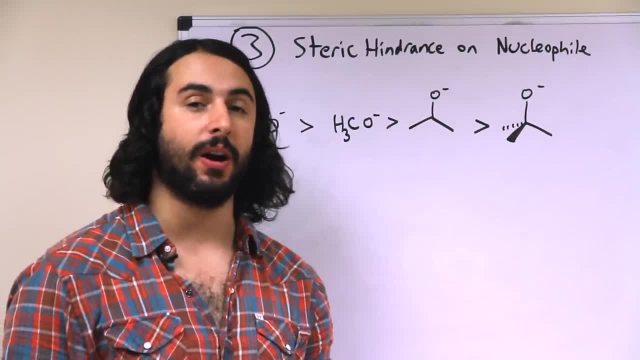 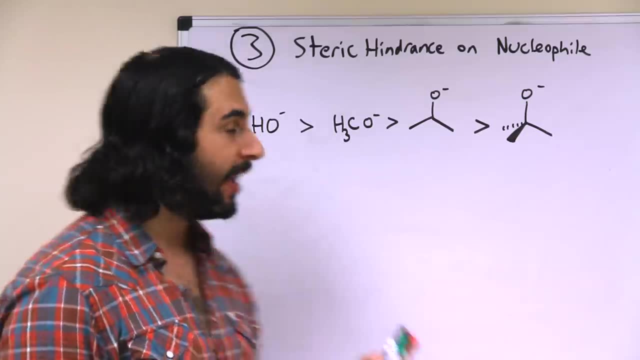 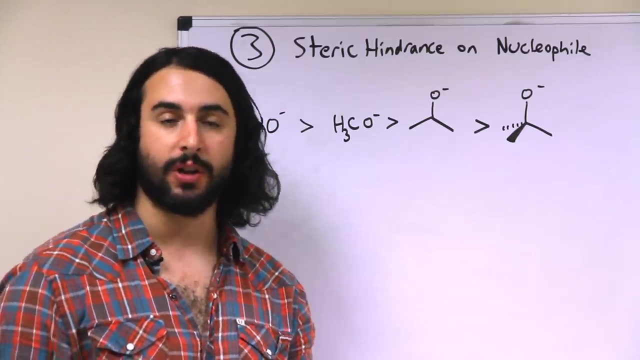 steric hindrance of the nucleophile and there is a point where a nucleophile will no longer be able to approach a substrate because of all the steric hindrance. and so hydroxide being very small, is able to approach even a, you know, a secondary system with, with some beta branching, doesn't really matter. 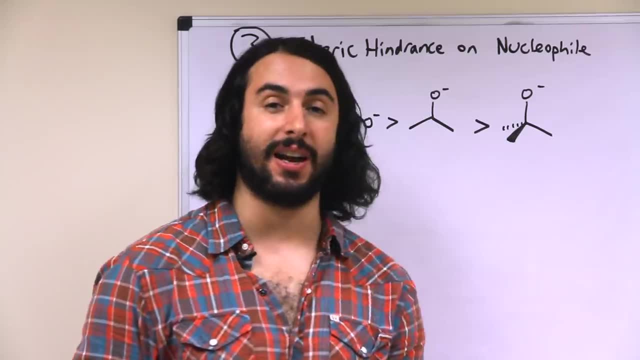 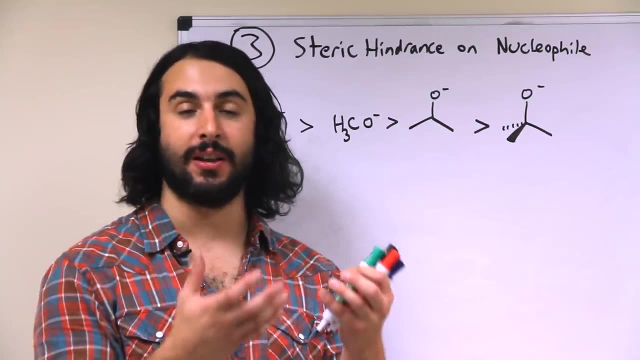 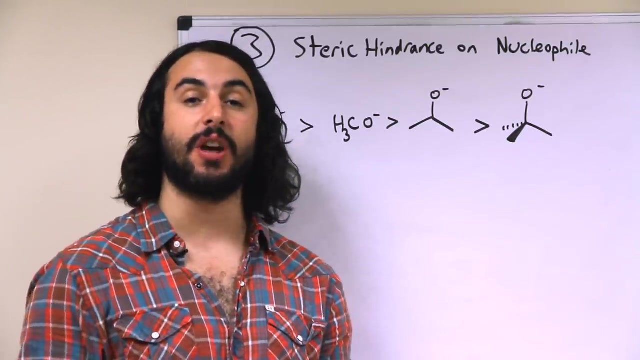 it's quite small. however, tert butoxide is the classic E2 promoter because it is simply too sterically hindered to approach the substrate and substitute. so the more sterically hindered the base, the less likely it is to substitute and the more 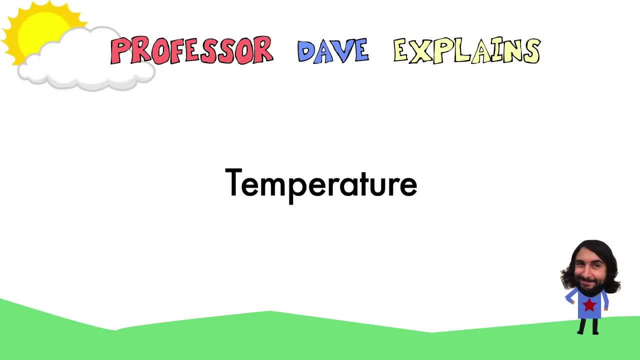 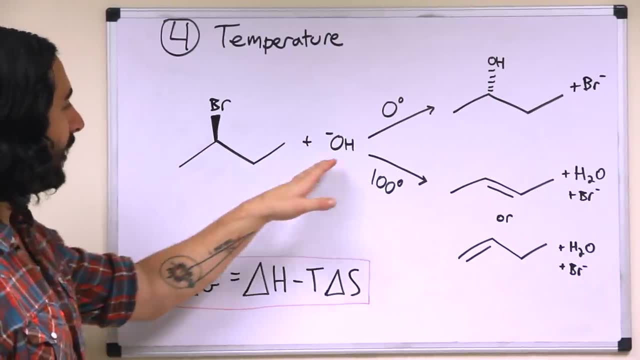 likely it is to eliminate. the last thing we want to look at is temperature. so let's take a system like this. we've got a secondary halo alkane. we've got hydroxide. hydroxide is very strong. we know we're probably looking at SN2 or E2, but we can look at. 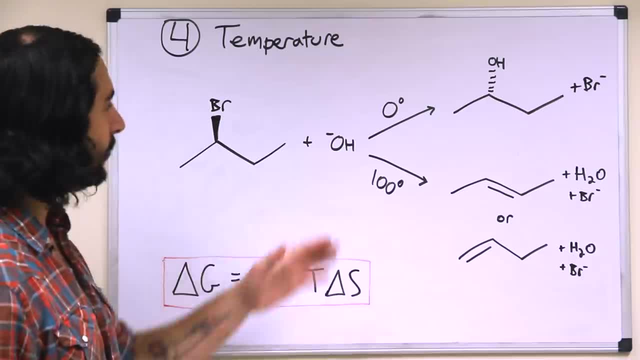 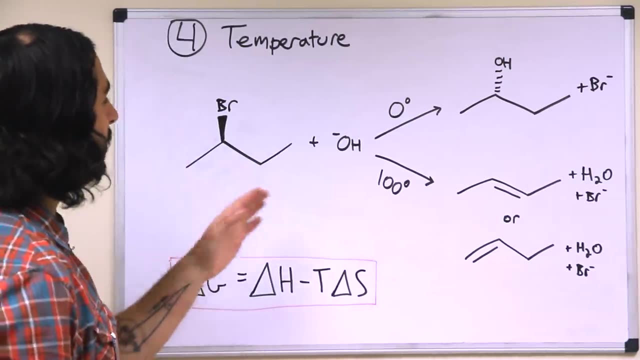 temperature to choose which one is going to occur. so let's take two hypothetical temperatures. let's call 0 a cold temperature and 100 is going to be our hot temperature. so, as it turns out, cold temperatures favor substitution. so at 0, it's much. 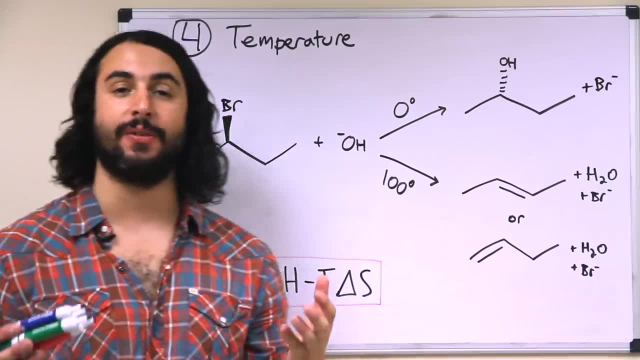 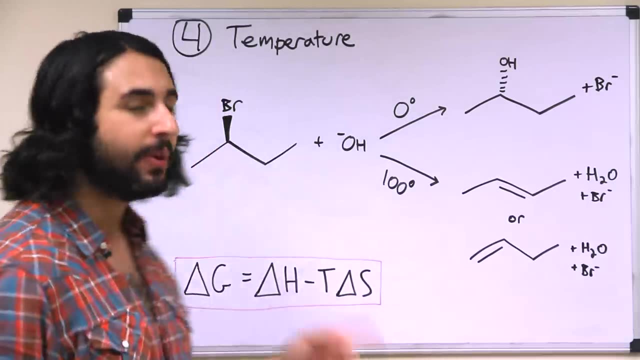 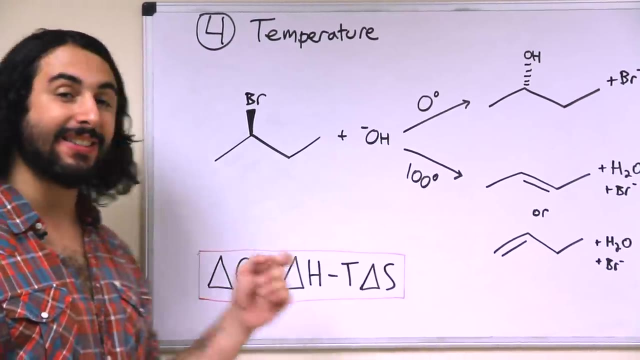 more likely to get the SN2 product, and hot temperatures favor elimination, so at 100 we're much more likely to get one of the two possible elimination products. now the reason for this lies in the Gibbs free energy equation, so hopefully we remember this from gen chem. so delta G equals delta H, minus T, delta S. so 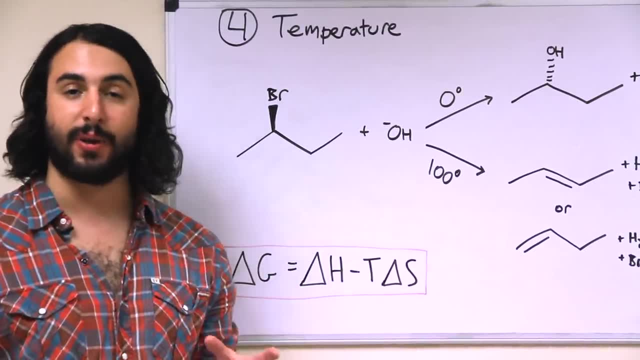 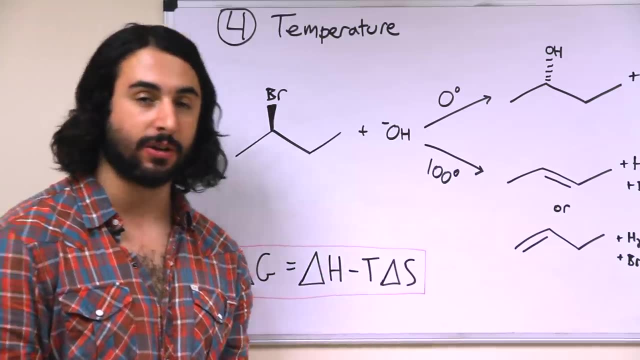 delta G is the term that it's Gibbs free energy. it refers to the spontaneity of any given reaction. so a negative value for delta G means it's going to be a spontaneous reaction. positive will be non-spontaneous delta H. 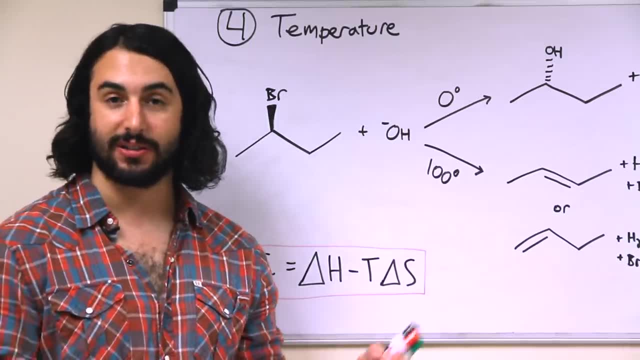 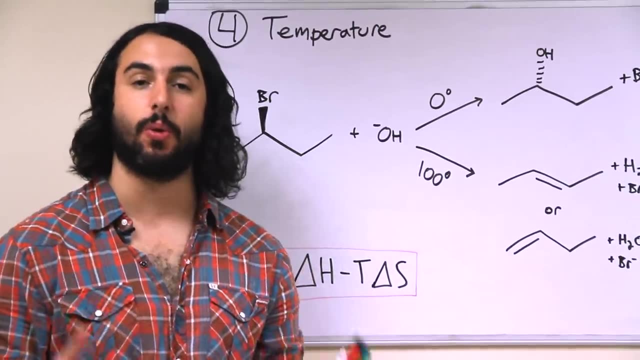 is the change in enthalpy. so that's basically energy, the energy that's associated with the change in the reaction. and then T is temperature delta, S is the change in entropy or disorder. so one thing we need to understand is that an elimination reaction is more entropically. 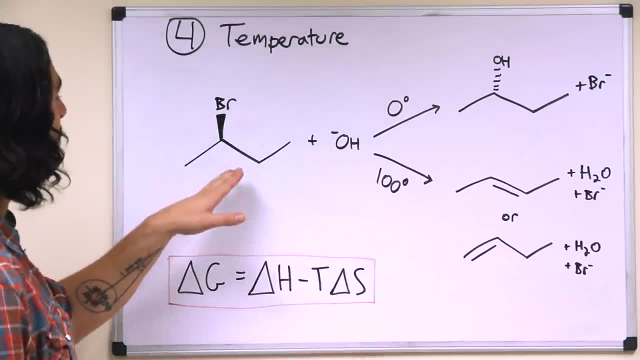 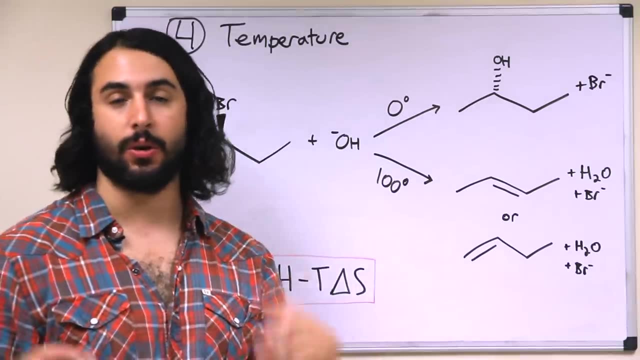 favorable than a substitution reaction. and here's why we have a substrate, a nucleophile, and we have a nucleophile, we have the product and the leaving group, so that's two molecules or atoms generating two things. so two things, two things. 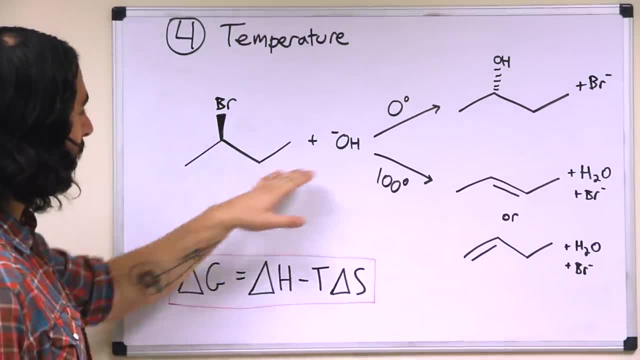 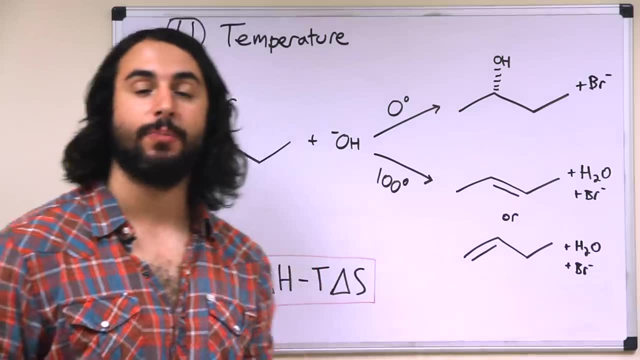 however, with an elimination. so we have the same setup at the start here. but look what happens at the end. we have the product, we have a water molecule and a bromide, so two things become three things: more disorder. that's entropically. 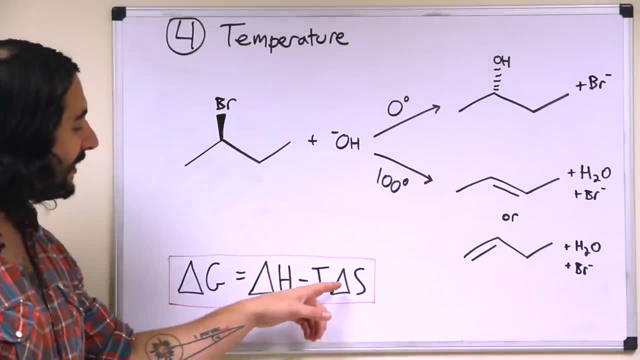 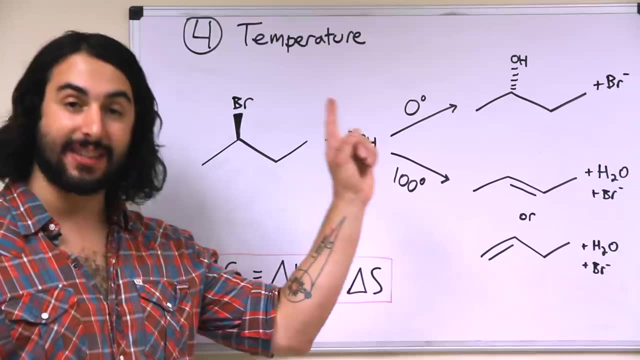 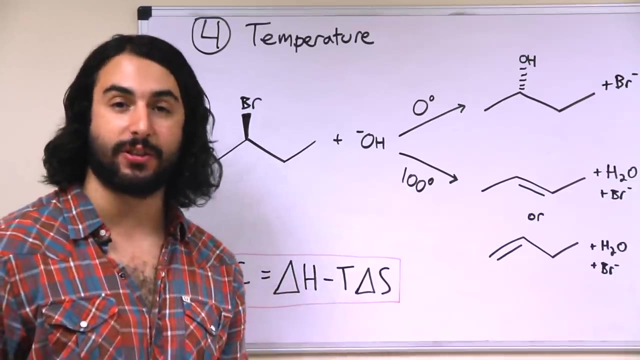 favorable. now the thing about the equation is that the change in entropy is being multiplied by temperature. so that means that at very high temperatures the entropic favorability or unfavorability becomes a greater factor in determining the spontaneity of the reaction. so let's say we have a very 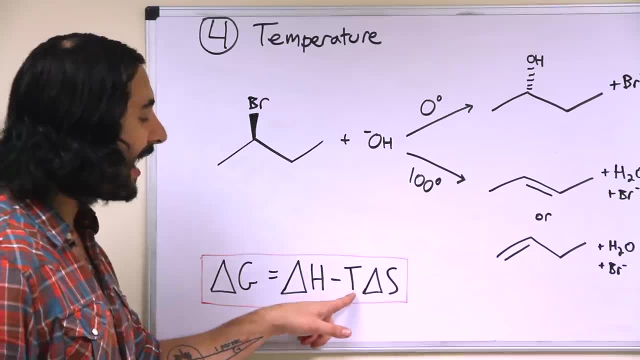 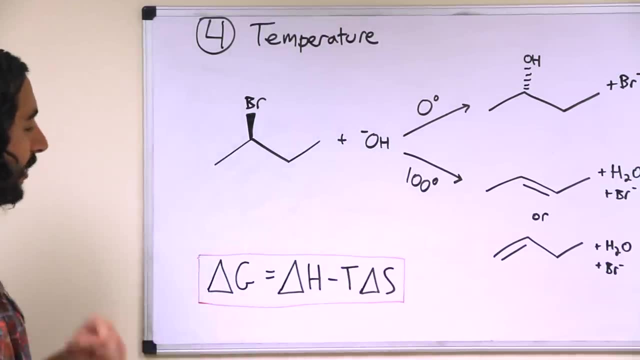 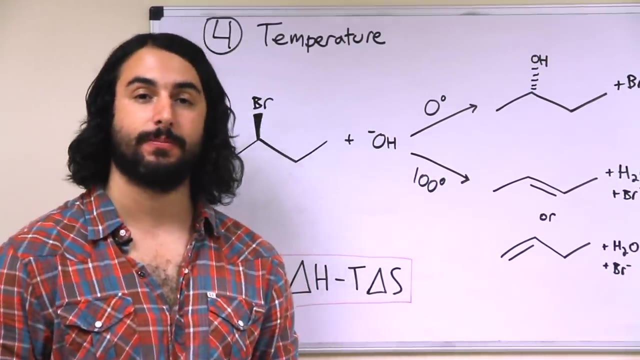 entropically favorable situation like an elimination at a high temperature, this whole T delta S term becomes more significant and it becomes more likely that delta G is going to end up having a negative value. so that's why, at high temperatures, elimination is going to be favored. so it 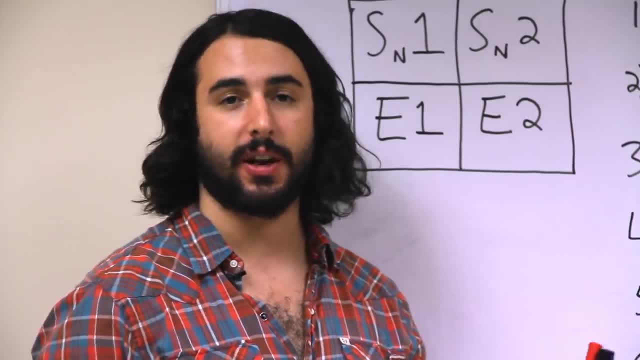 can be tricky to choose which mechanism is occurring, but as long as we look at the substrate and the nucleophile, we ought to be able to eliminate some options. so let's put it all together and look at some examples, if we're going to 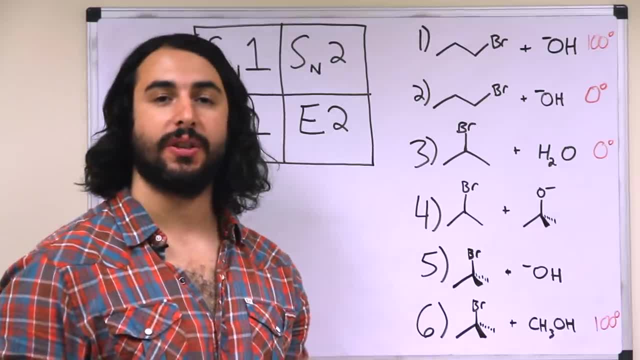 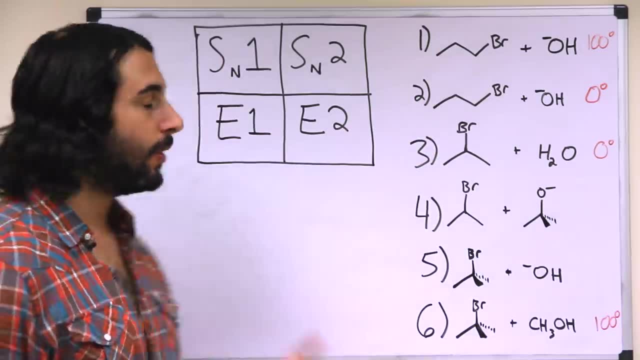 look at something like this. so the first thing we can do is look at the substrate and see if we can eliminate any of the possible mechanisms. so this is a primary halo alkane. so immediately we can get rid of S and 1 and E1.. we're not going to form that primary carbocation: S and 1 and E1, both. 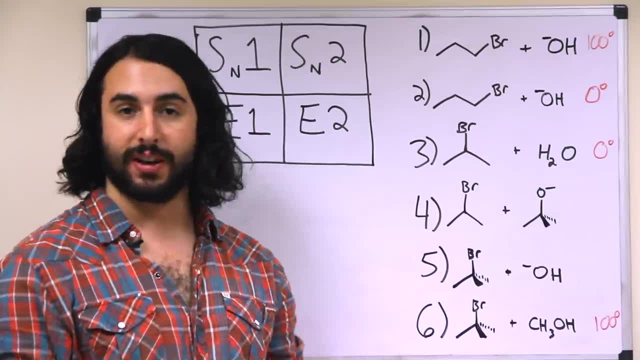 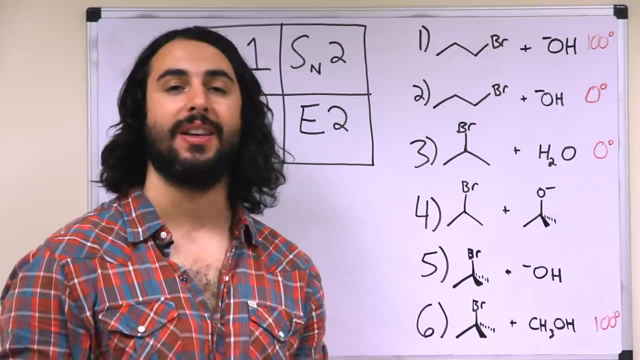 require a carbocation intermediate to occur. so we're going to get rid of those options. we know it's going to be SN2 or E2.. likewise, if we look at the strength of the base, that's a strong base, it's a strong nucleophile. it doesn't have to. 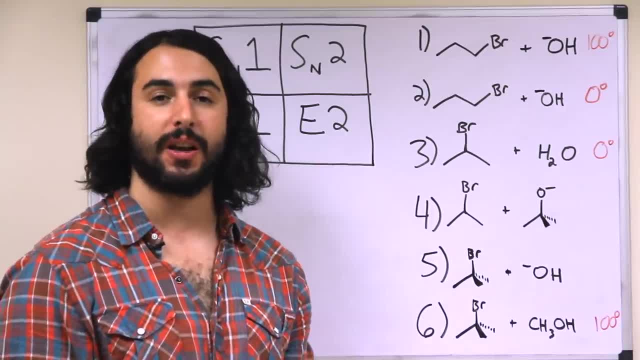 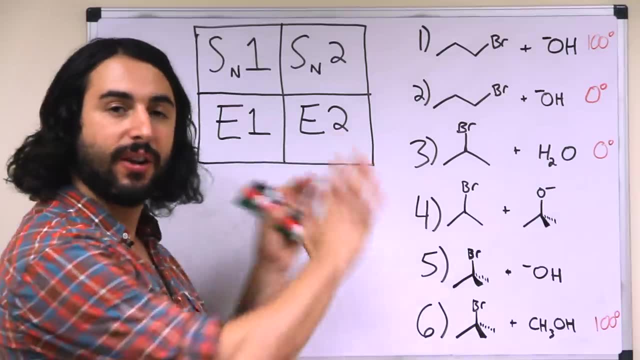 wait for a carbocation to occur. it can bully around a substrate and make a reaction happen. so by that reasoning, again we're looking at SN2 or E2.. so we've just gotten rid of half of the options and now we're down to SN2 and E2. 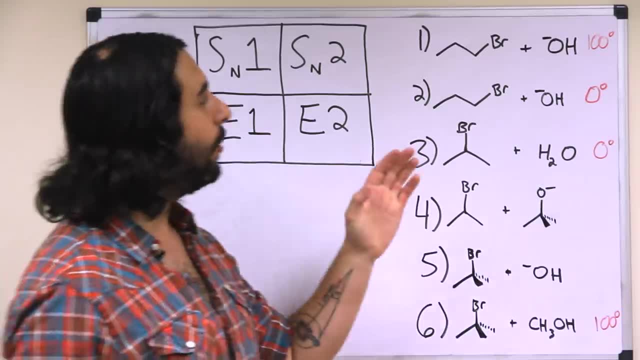 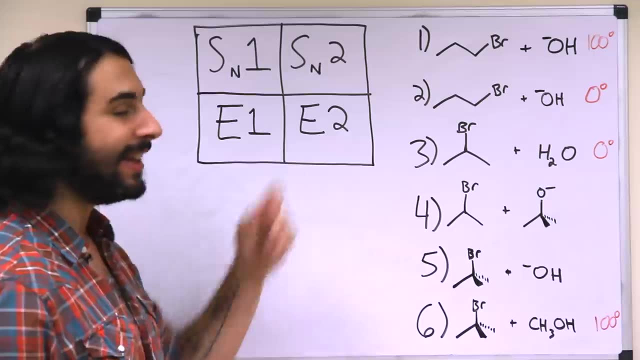 just from looking at that substrate and the base. so between SN2 and E2 we might have to look at maybe a temperature. let's say we're doing this at a hundred degrees- that is going to cause us to favor E2, because hot temperatures favor elimination. so number 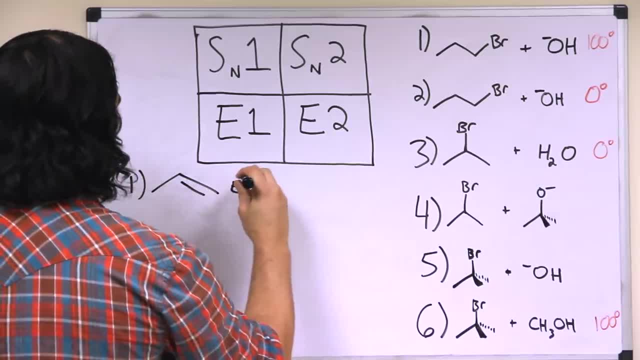 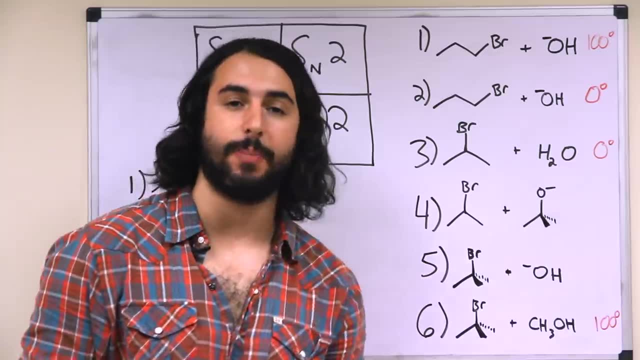 one. we're going to go with that as our E2 product. okay, so number two: same setup, right, but both by looking at the substrate and the base, both of those things are telling us that we're looking at SN2 or E2. again, now we're looking at 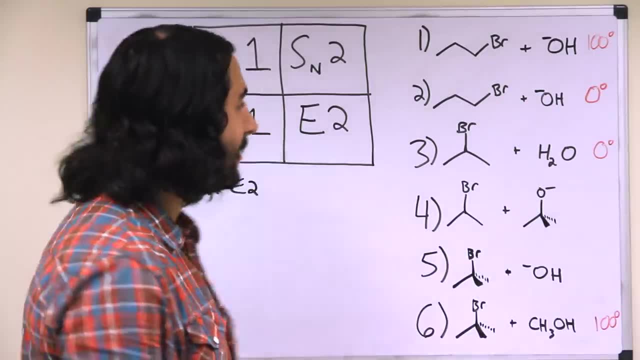 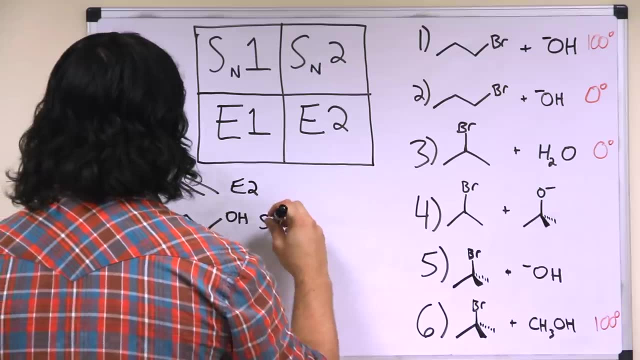 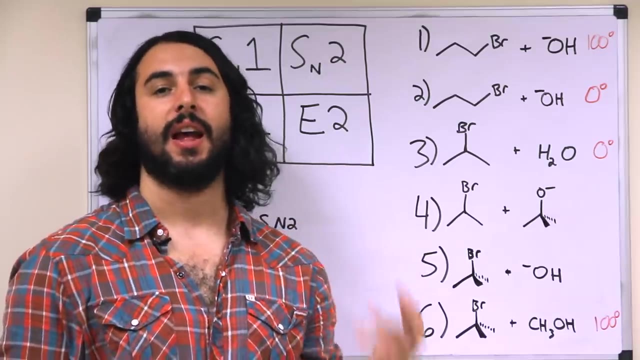 the cold temperature. this time maybe we're going to favor some SN2.. so number two: we're looking at that as our most likely product, SN2.. so again, we're looking at the substrate, we're looking at the strength of the base and we're 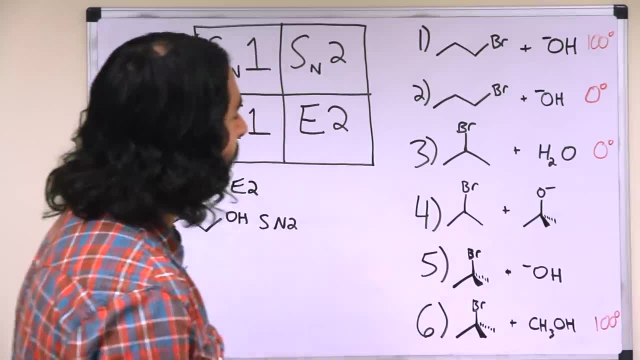 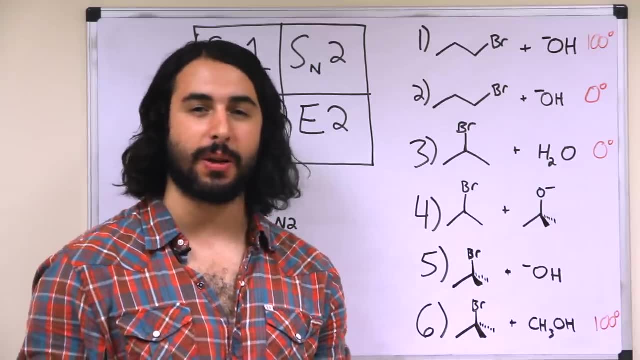 looking at the temperature that's going to get allow us to figure out what's going on. so let's look at this one. now. we have a secondary substrate, so with the secondary halo alkane, we're not really going to be able to figure out. 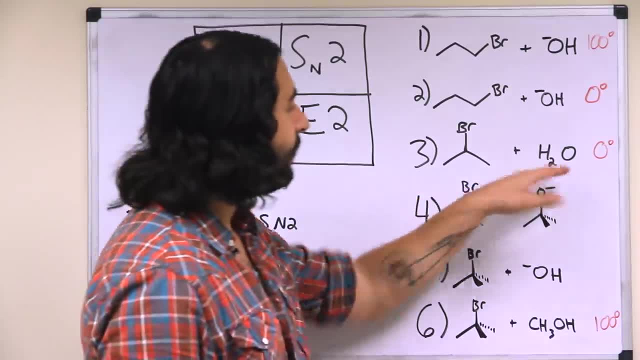 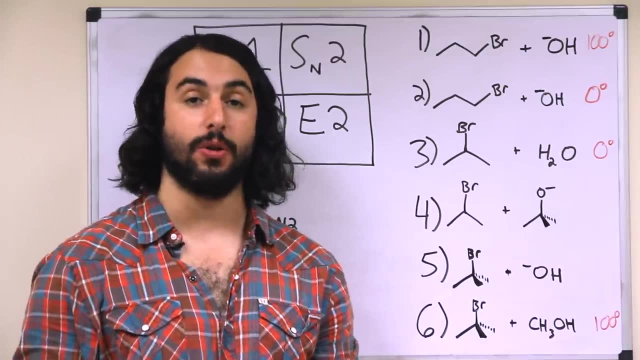 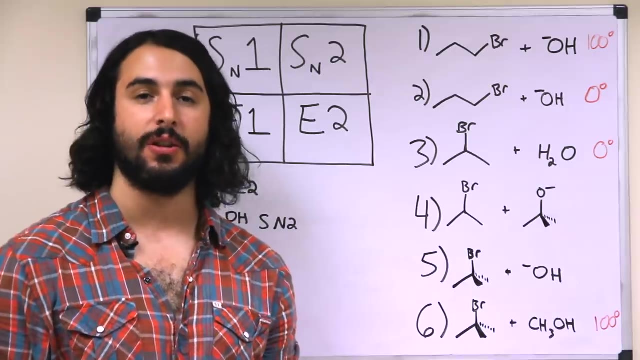 too much about which reactions are going to happen or which mechanism is going to occur, but we're looking at water as the nucleophile. so water is a weak base, so it is a poor nucleophile. that means we can get rid of Sn2 and E2 as possibilities, because it's not a strong enough nucleophile to do. 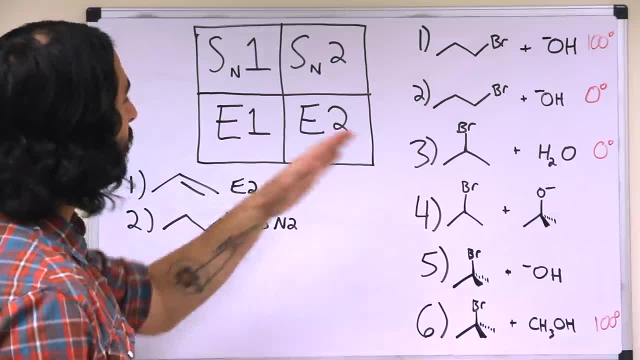 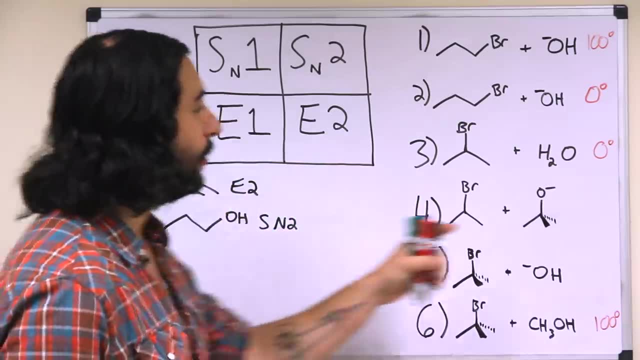 either of those reactions, either of those mechanisms. so we know we're going to get Sn1 or E1, okay, now between the two we can look at the temperature again. this time let's say zero. so that means we're going to favor Sn1, because 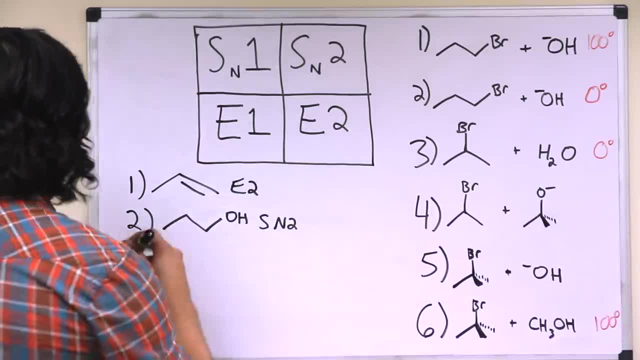 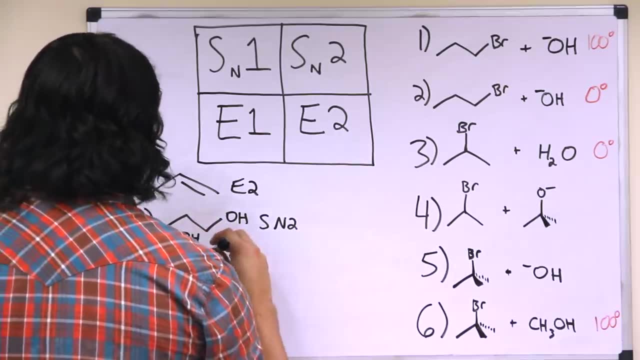 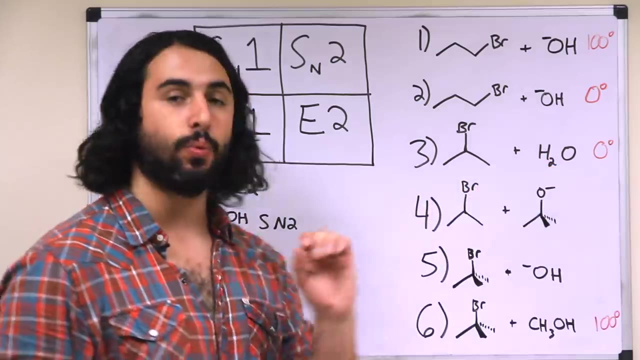 colder temperatures favor substitutions. so we know that we're going to be looking at this and that is our Sn1 product, okay. so once again, we're just looking at the base and we're seeing that that is weak. that is a weak nucleophile, and a weak nucleophile will not be able to do Sn2 or E2, so we're. 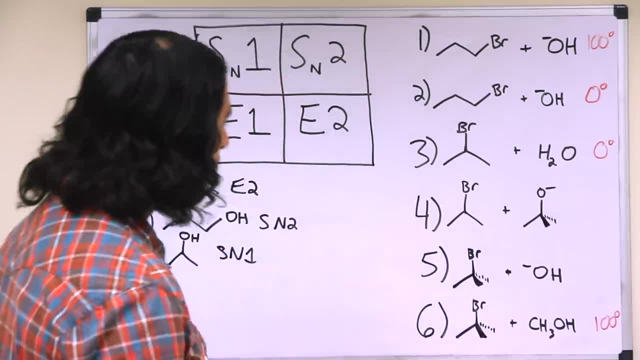 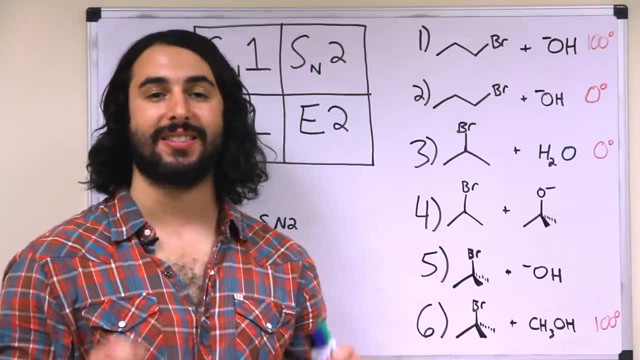 getting rid of those possibilities. and then we look to the temperature. so how about this? we've got the same substrate. now we've got that tert butoxide. so if we remember from before, tert butoxide is the classic E2 promoter. now, the reason for this is it is strong. 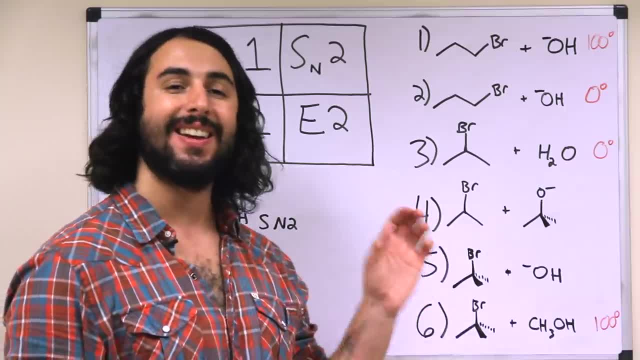 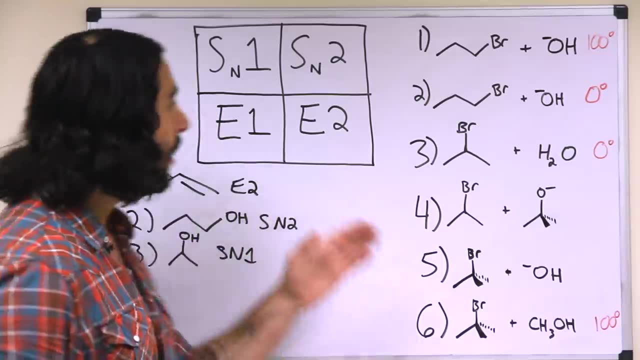 it is an alkoxide. it is a. it has a formal negative charge. so alkoxides are strong bases. so a strong base is a strong nucleophile. so it's going to be able to do SN2 or E2. it does not need to wait for a carbocation. it's gonna. it's. 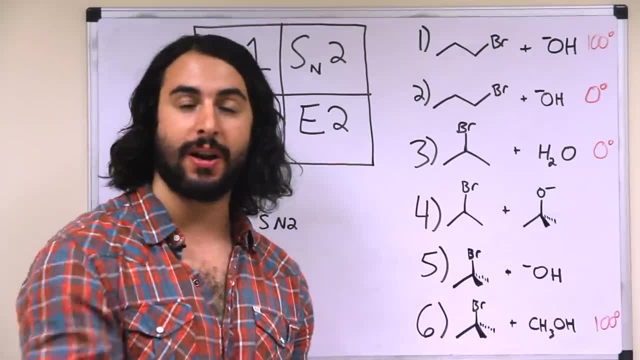 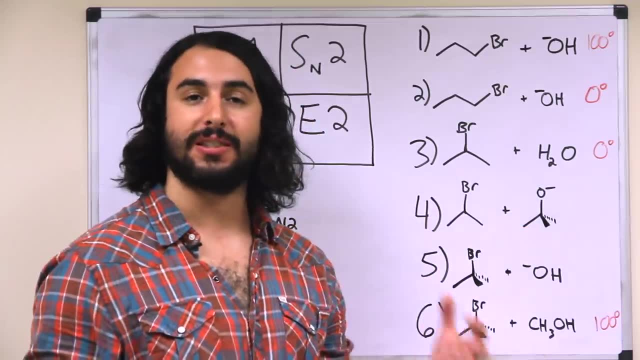 gonna make something happen. it sees this substrate and it's either going to try to coordinate or is going to do an acid-base reaction because it's a strong base. now the thing is that- remember before we were talking about steric hindrance of the nucleophile- there is too much steric hindrance associated. 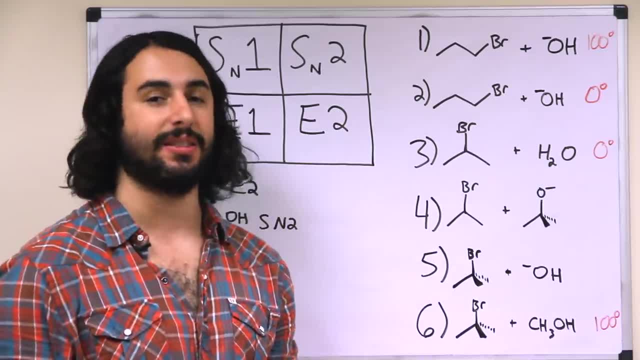 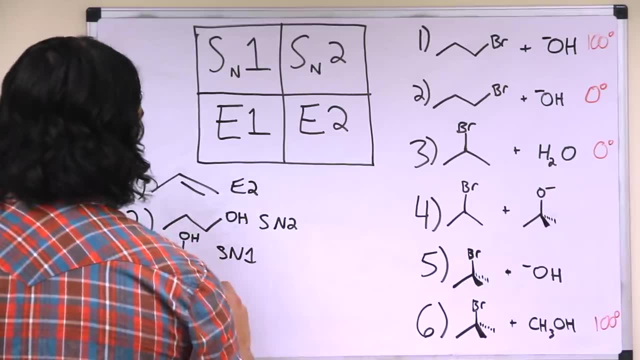 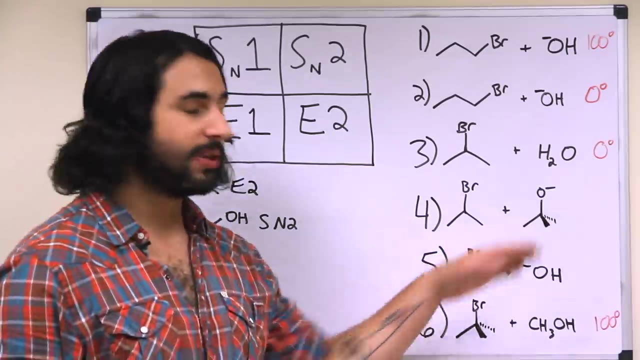 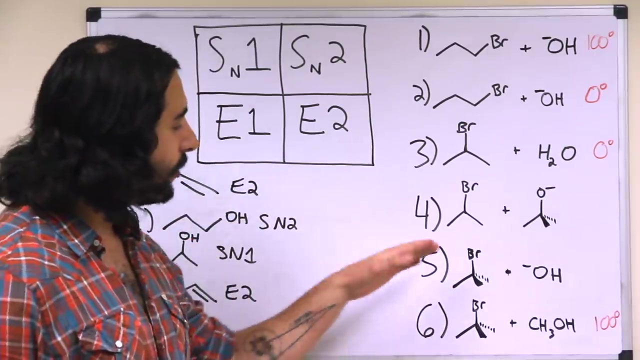 with this nucleophile for it to coordinate. it cannot do SN2, so this can only do E2. so there is our E2 product. okay. so remember tert butoxide always gonna go E2. so now let's look at a tertiary halo, alkane. so with the tertiary, we can remember we're gonna. 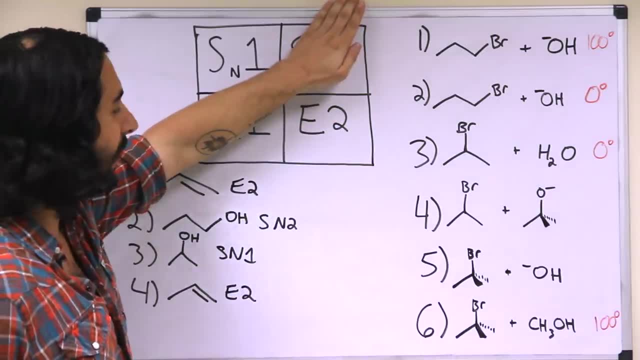 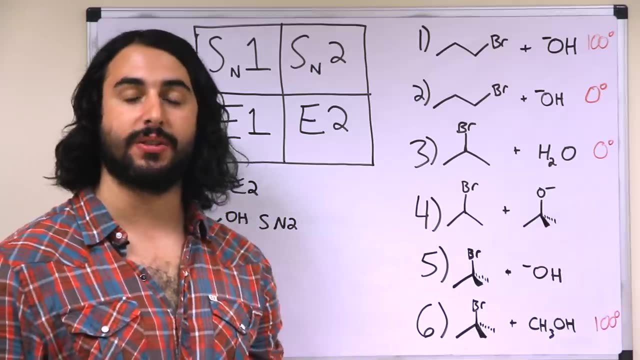 we're not going to be able to do SN2, so we're getting ready, we're getting rid of that possibility. now the thing is: hydroxide is strong. hydroxide is a strong base, so it's a strong nucleophile, so it's able to do SN2 or E2. it doesn't. 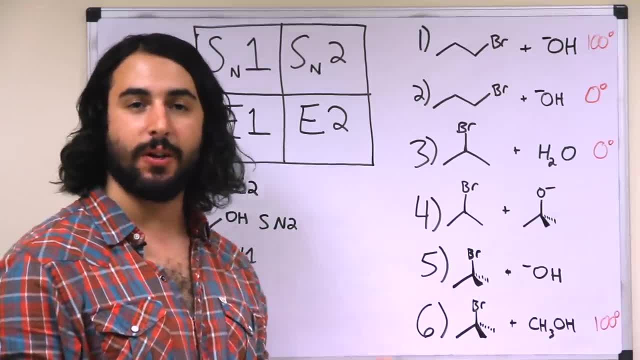 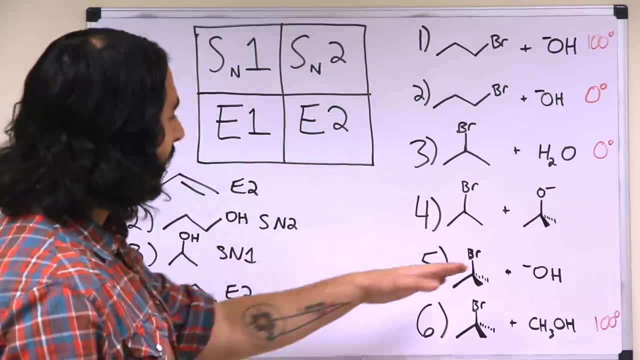 need to wait for a carbocation to form, so SN1 and E1 aren't gonna happen. that's just gonna take too long. hydroxide finds a substrate and solution. it's gonna bully it around, it's gonna do something, but we just said it can't do SN2, so the only possibility is therefore: 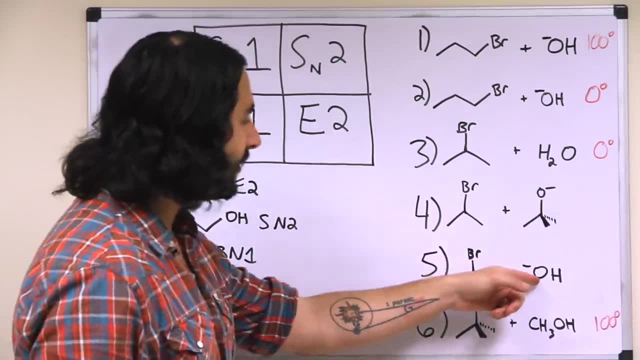 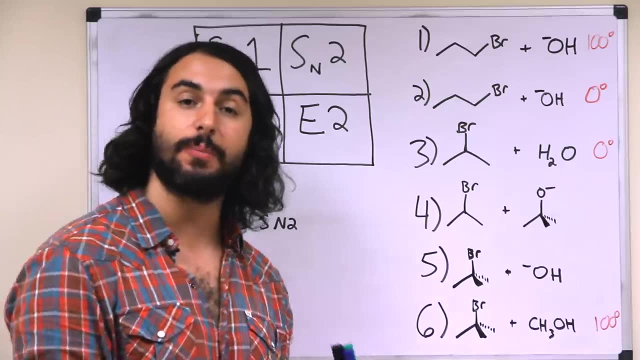 E2. we don't even have to look to a temperature. we're seeing that this is gonna want to either substitute or eliminate. it cannot substitute because of the steric hindrance associated with the substrate this time. so that is going to give us an E2 product. 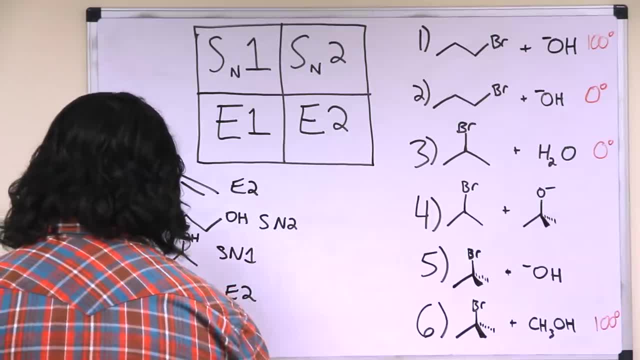 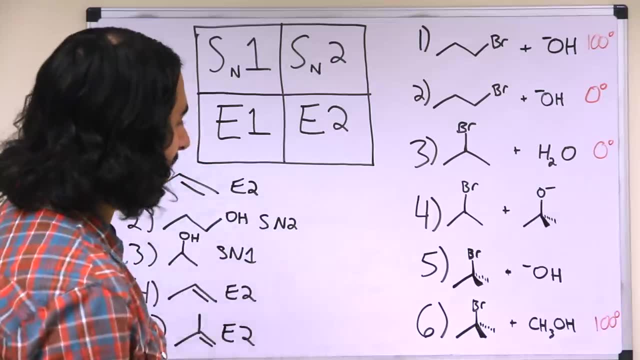 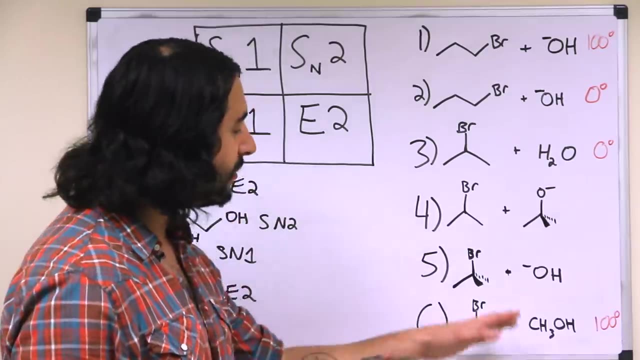 so number five: we added a little bit of E2 here, added a carbon this time. so there's that. so there is our E2 product, incapable of doing SN2. now, same substrate. now we're looking at methanol now. so methanol is weak, right. there is no formal charge there. it is, it is. 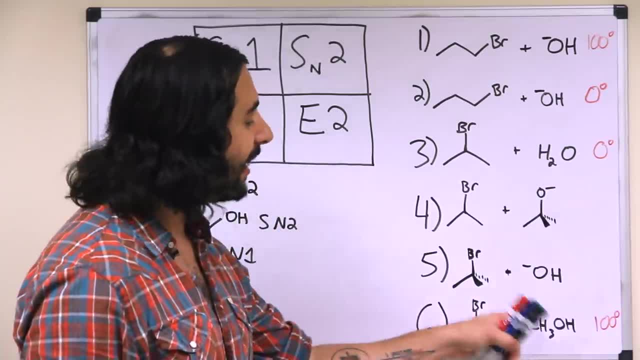 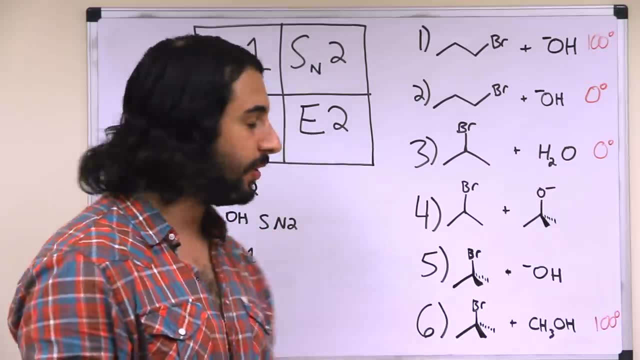 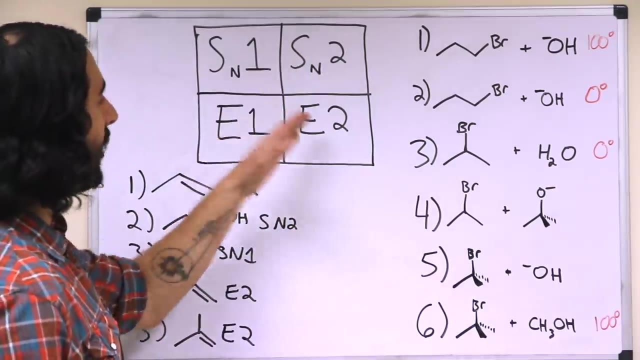 comparable to water in terms of basicity, just has that extra methyl group instead of a hydrogen, but it's completely covalent. there's no, it's neutral. there's no negative charge. so that is a weak base, so it is a poor nucleophile, so it is not strong enough to do SN2 or E2. 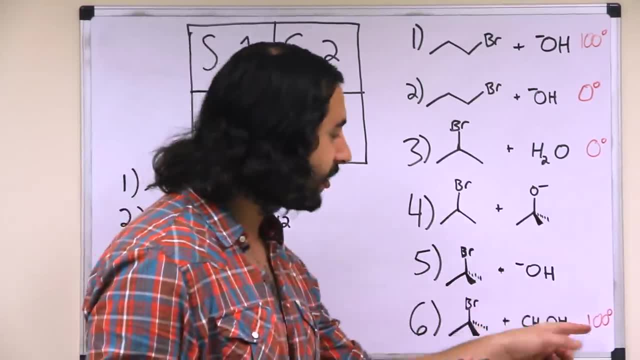 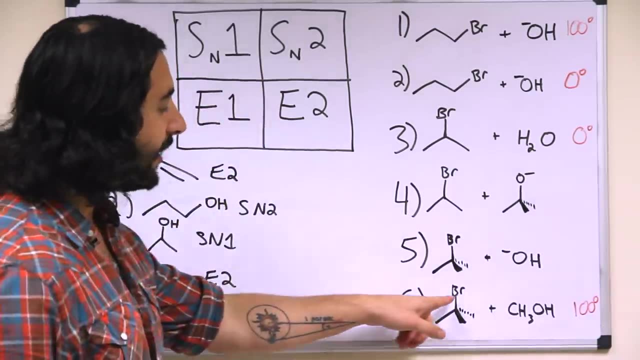 so it's gonna be SN1 or E1. we're gonna look at the temperature: hundred degrees once again. that favors elimination, so. but it is weak so it's gonna do E1. so it has to wait for that bromine to leave. once that bromine leaves and we have the 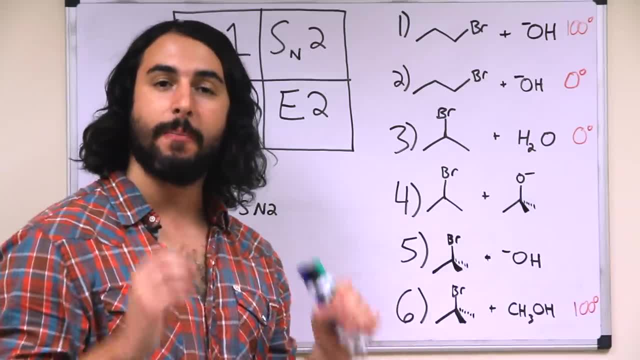 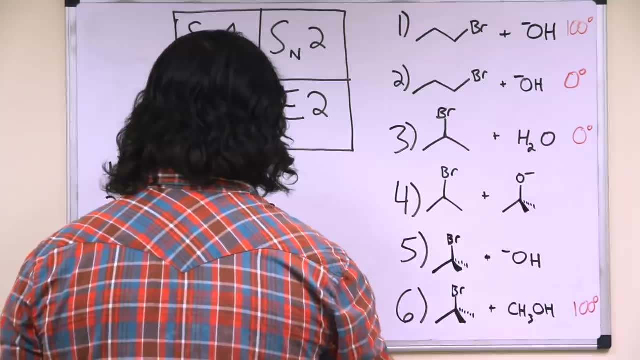 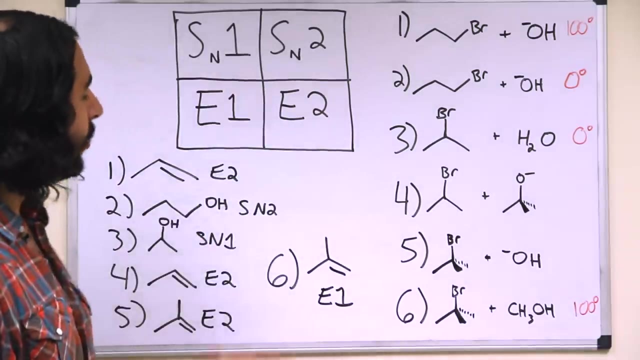 carbocation, then those beta protons become much, much more acidic, such that even a weak base like methanol is going to be able to extract one. so let's say, number six is our E1 product. okay, so here's a few examples and we're able to see how each mechanism could be.